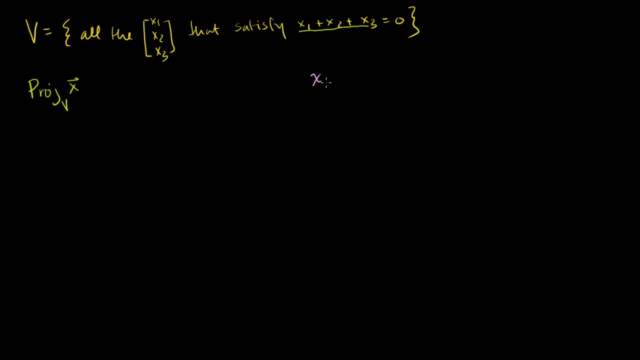 Let's say that x2 and x3 are kind of free variables and we could say x1 is equal to minus x2, minus x3. And then let's just just so that we can write it in kind of our parametric form, or if we can write our solution, set as the combination of basis vectors, we can say x2 is equal to, let's say it's equal to, some arbitrary constant, c2.. 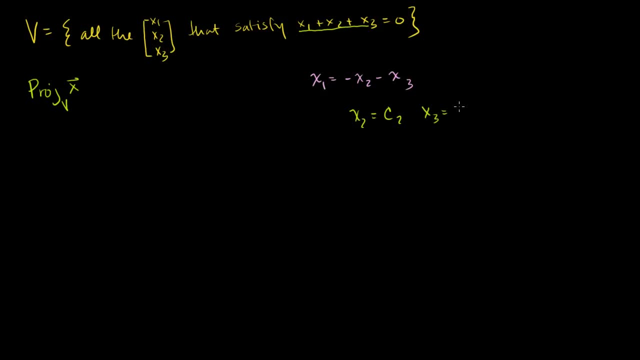 And let's say that x3 is equal to some arbitrary constant, c2. Then we can say that. then we can say that V, we can rewrite V. we can say that V is- I'll do it here- V is equal to the set of all x1s, x2s and x3s that are equal to c2 times. so x1 is equal to minus. let me write, let me rewrite this, let me rewrite this with the c2s. 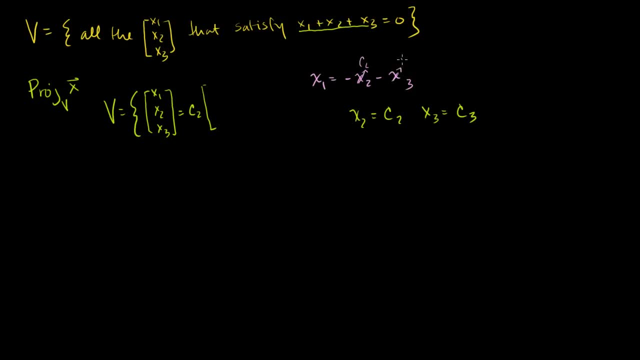 This is equal to c2.. This is equal to c3.. So x1 is equal to minus c2 minus c3.. So x1 is equal to minus 1 times c2 plus c3 times what, Plus c3 times minus 1.. 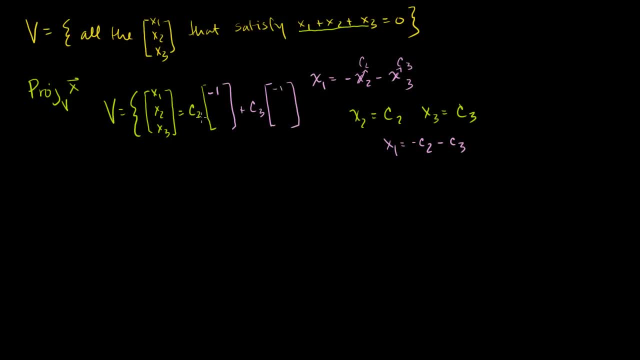 And then what is x2 equal to? x2 is just equal to c2.. So it's 1 times c2 plus 0 times c3.. x3 is just equal to c3.. So it's 0 times c3.. 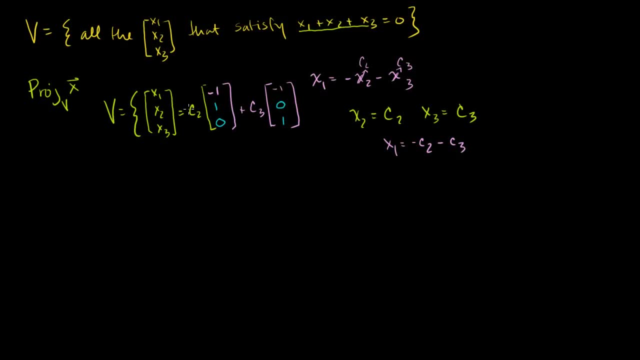 c2 plus 1 times c3.. And so this is another way of defining our subspace. All of the vectors that satisfy. this is equal to is equal to this definition here, It's all the vectors whose components satisfy or that lie in this plane, whose entries lie in that plane. 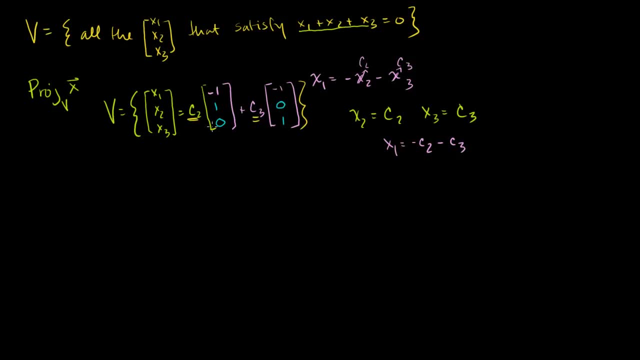 And that's for any real numbers right there, Or another way of writing that, another way of writing this is that V is equal to the span. V is equal to the span of the vectors minus 1,, 1, and 0.. 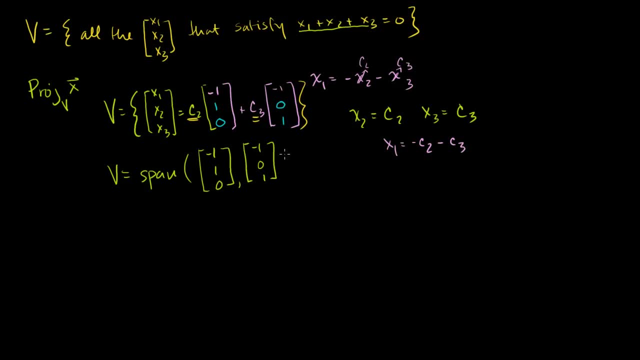 And the vector minus 1, 0, and 1.. Just like that. And we know that these are actually a basis for V because they're linearly independent. There's no way I can take linear combinations of this guy and make the second entry be equal to 1 here. 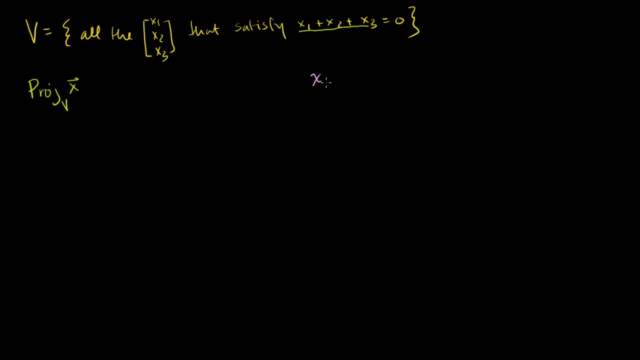 Let's say that x2 and x3 are kind of free variables and we could say x1 is equal to minus x2, minus x3. And then let's just just so that we can write it in kind of our parametric form, or if we can write our solution, set as the combination of basis vectors, we can say x2 is equal to, let's say it's equal to, some arbitrary constant, c2.. 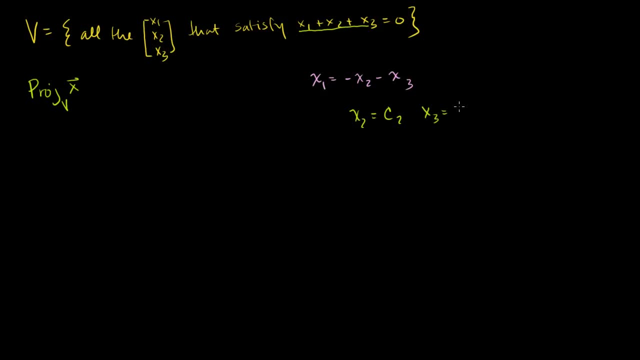 And let's say that x3 is equal to some arbitrary constant, c2. Then we can say that. then we can say that V, we can rewrite V. we can say that V is- I'll do it here- V is equal to the set of all x1s, x2s and x3s that are equal to c2 times. so x1 is equal to minus. let me write, let me rewrite this, let me rewrite this with the c2s. 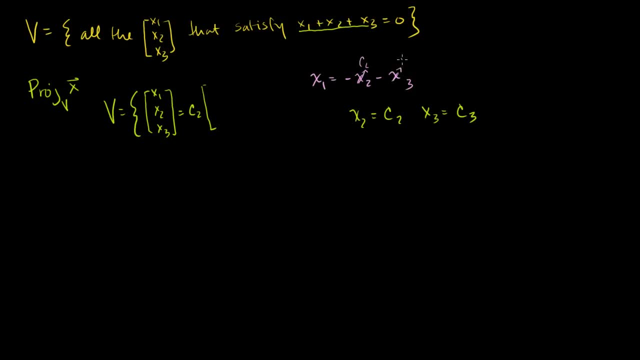 This is equal to c2.. This is equal to c3.. So x1 is equal to minus c2 minus c3.. So x1 is equal to minus 1 times c2 plus c3 times what, Plus c3 times minus 1.. 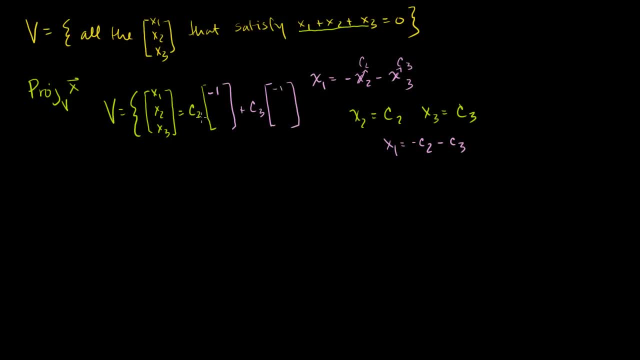 And then what is x2 equal to? x2 is just equal to c2.. So it's 1 times c2 plus 0 times c3.. x3 is just equal to c3.. So it's 0 times c3.. 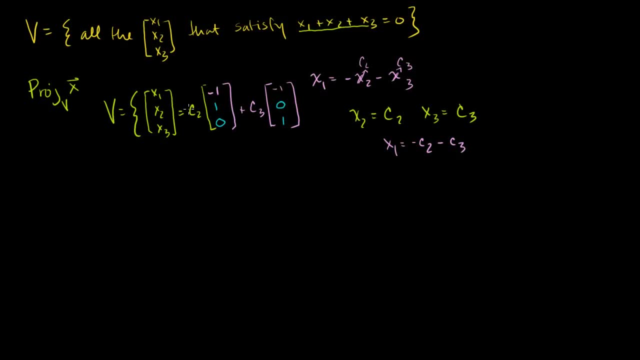 c2 plus 1 times c3.. And so this is another way of defining our subspace. All of the vectors that satisfy. this is equal to is equal to this definition here, It's all the vectors whose components satisfy or that lie in this plane, whose entries lie in that plane. 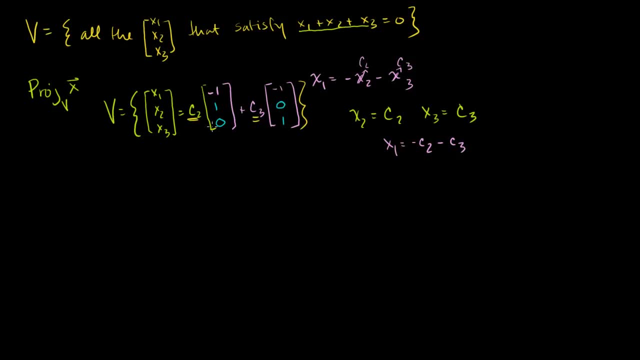 And that's for any real numbers right there, Or another way of writing that, another way of writing this is that V is equal to the span. V is equal to the span of the vectors minus 1,, 1, and 0.. 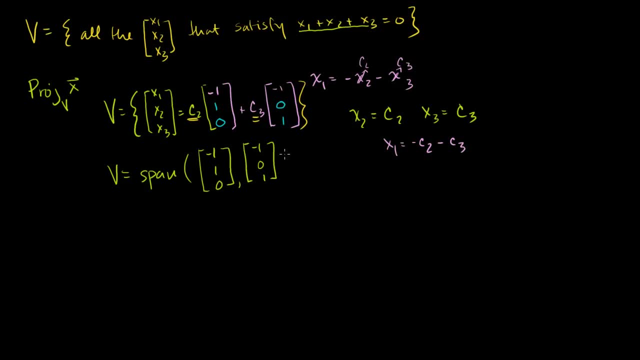 And the vector minus 1, 0, and 1.. Just like that. And we know that these are actually a basis for V because they're linearly independent. There's no way I can take linear combinations of this guy and make the second entry be equal to 1 here. 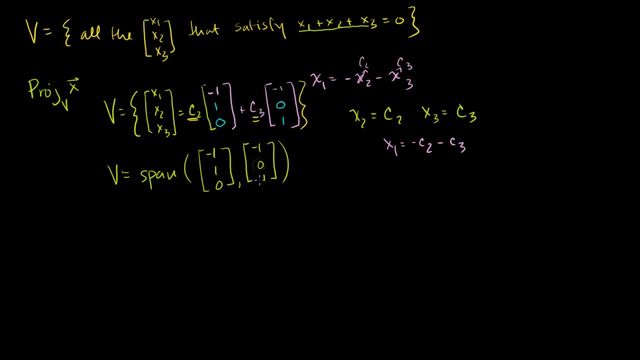 And likewise there's no way I can take linear combinations of this guy and make this third entry equal to 1 here. So these are also a basis for V. So given that just using the technique we did before, We could set some vector, we could set some matrix: A equal to minus 1, 1, 0.. 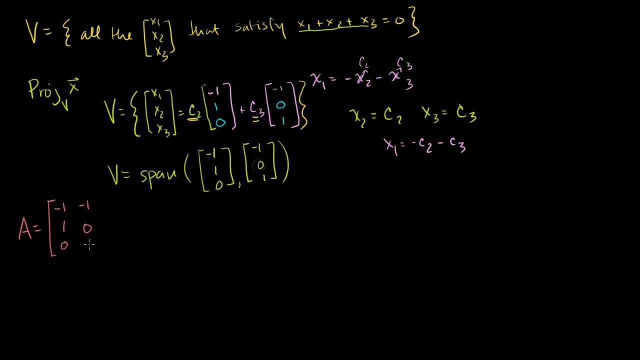 And then minus 1,, 0, and 1.. And then we can figure out. we can figure out that the projection of any vector x in R3. Onto V is going to be equal to- And we saw this is going to be equal to A. 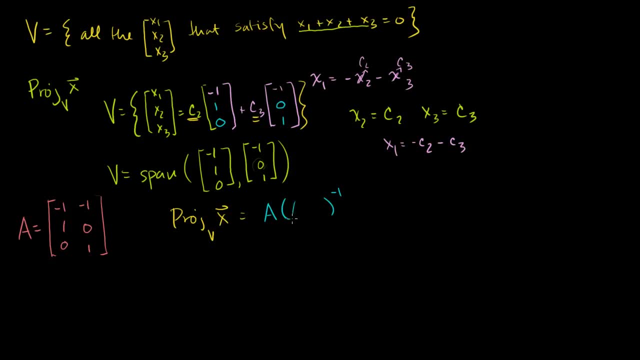 Times the inverse of A transpose A. All of that times A transpose, And all of that times x, And you can do it. You have A here. You can figure out what the transpose of A is Very easy. You can take A, transpose A. 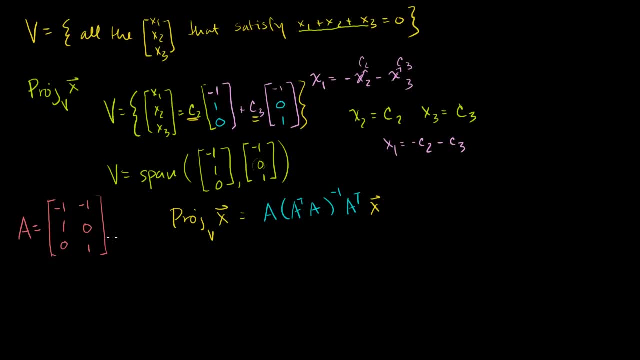 Then you can invert it And it'll be very similar to what we did in the last video. It'll be a little less work Because this is a 3 by 2 matrix Instead of a 4 by 2 matrix, But you saw. 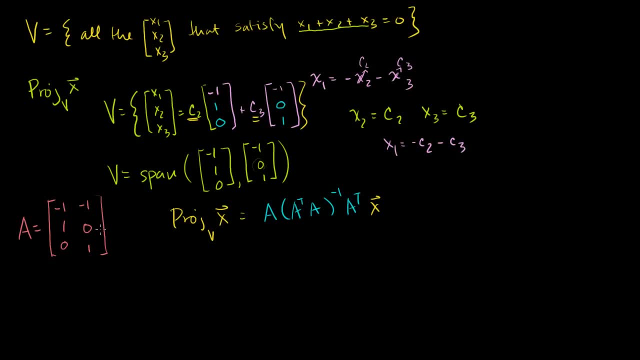 It is actually a lot of work. It's very hairy And you might make some careless mistakes. So let's think, Let's figure out if there's another way that we can come up. There's another way that we can come up with this matrix right here. 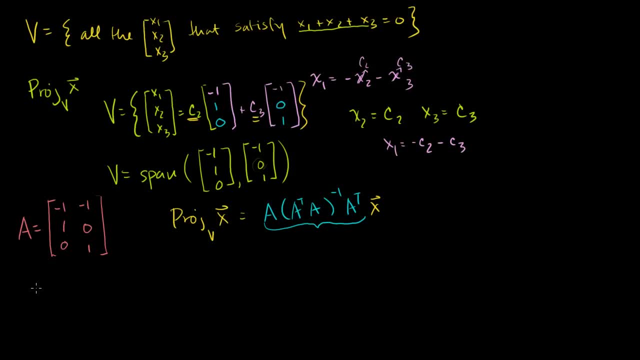 Now we know that if x is a member, We know that if x is a member of R3. That x can be represented. Then x can be represented As a combination of some vector v That is in our subspace, Plus some vector w. 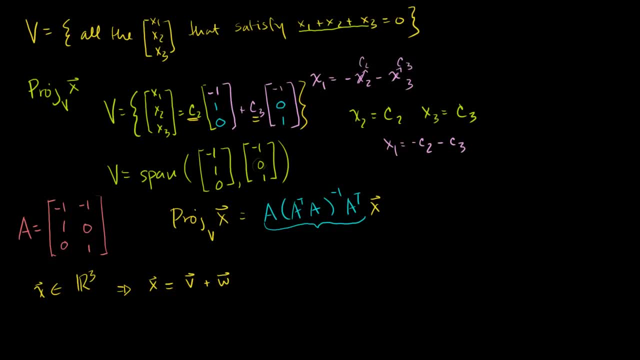 That is, in the orthogonal complement to the subspace, Where v is a member of our subspace And w is a member of the orthogonal complement, The orthogonal complement of our subspace. Now, by definition, This is That, right there. 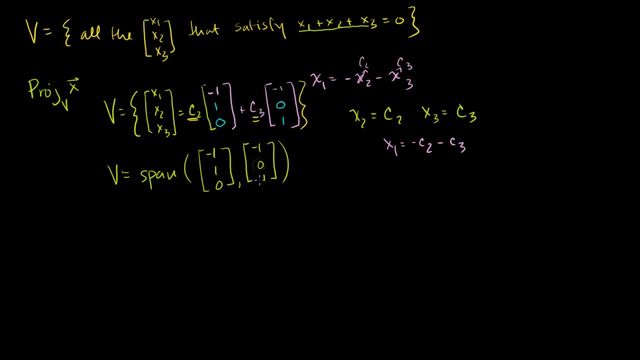 And likewise there's no way I can take linear combinations of this guy and make this third entry equal to 1 here. So these are also a basis for V. So given that just using the technique we did before, We could set some vector, we could set some matrix: A equal to minus 1, 1, 0.. 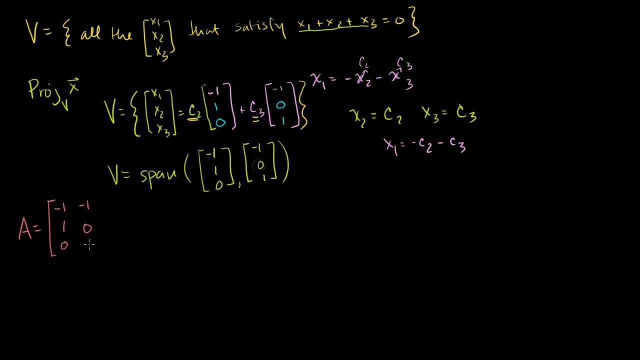 And then minus 1,, 0, and 1.. And then we can figure out. we can figure out that the projection of any vector x in R3. Onto V is going to be equal to- And we saw this is going to be equal to A. 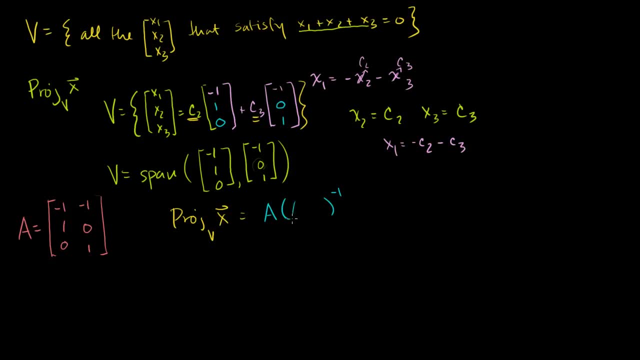 Times the inverse of A transpose A. All of that times A transpose, And all of that times x, And you can do it. You have A here. You can figure out what the transpose of A is Very easy. You can take A, transpose A. 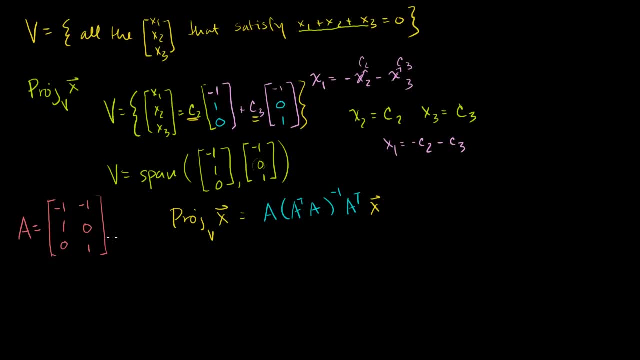 Then you can invert it And it'll be very similar to what we did in the last video. It'll be a little less work Because this is a 3 by 2 matrix Instead of a 4 by 2 matrix, But you saw. 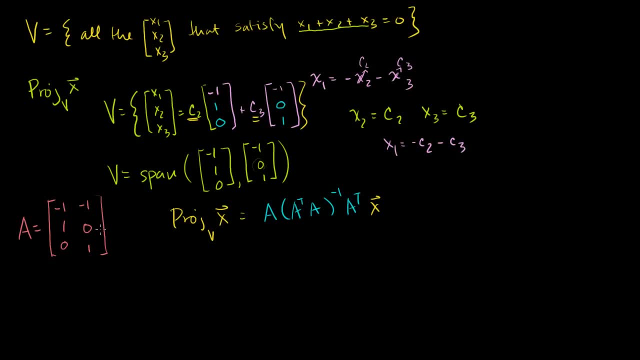 It is actually a lot of work. It's very hairy And you might make some careless mistakes. So let's think, Let's figure out if there's another way that we can come up. There's another way that we can come up with this matrix right here. 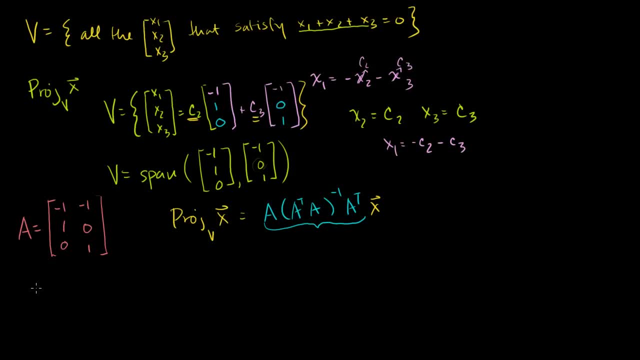 Now we know that if x is a member, We know that if x is a member of R3. That x can be represented. Then x can be represented As a combination of some vector v That is in our subspace, Plus some vector w. 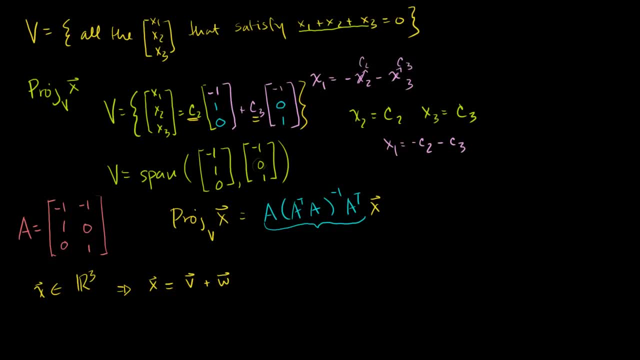 That is, in the orthogonal complement to the subspace, Where v is a member of our subspace And w is a member of the orthogonal complement, The orthogonal complement of our subspace. Now, by definition, This is That, right there. 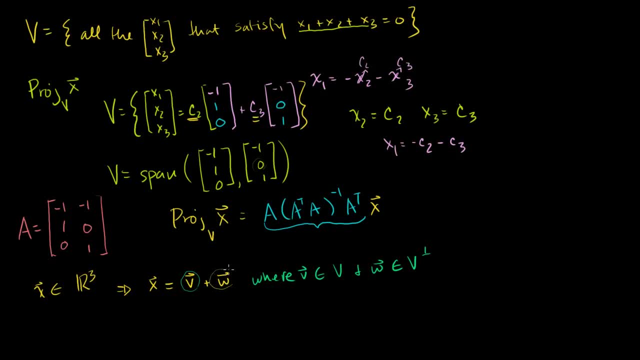 Is the projection of x onto v And this is the projection of x onto the orthogonal complement of v. So we can write that x- x is equal to the projection onto v of x Plus the projection onto v's orthogonal complement Of x. 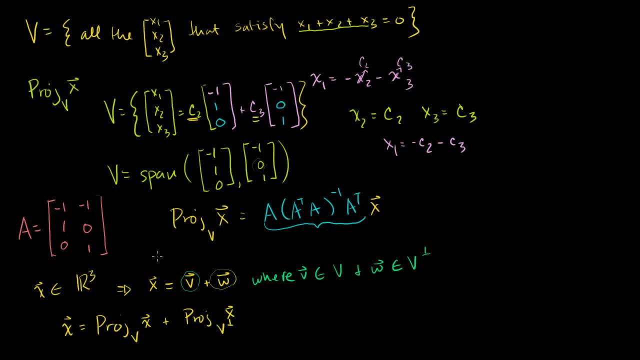 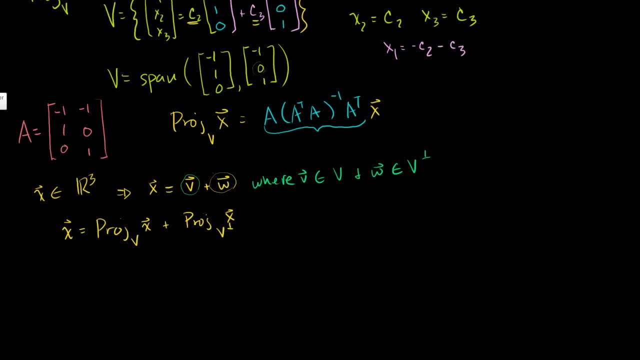 So this is by definition That any member of R3 can be represented this way. Now, if we want to write this as matrix vector products, In two videos ago I showed you that these are linear transformations, So let me write that here. 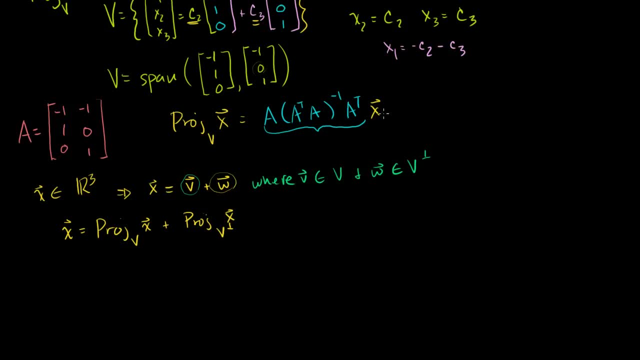 So they're linear transformations, So they can be written as matrix vector products. You see that, right there, Let me define this matrix. I don't know, Let me call this, Let me call this. I don't know, Let's just call this matrix. 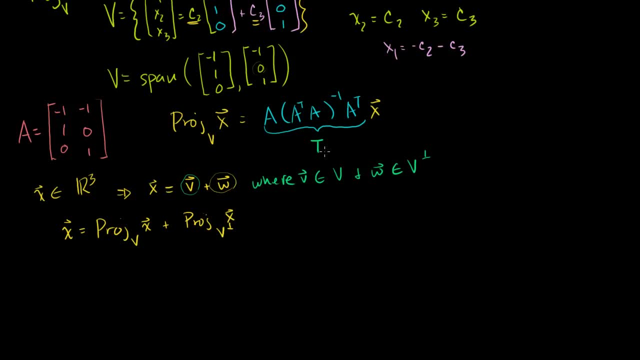 T, T, Let me just call it T And let me call. Let me call, Let me do another, Let me do a letter, Let me do b And let's say that the projection, The projection of Onto the orthogonal complement of v. 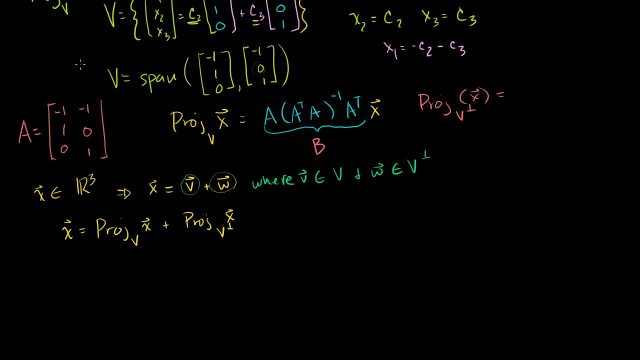 Of x, Let's say that that's equal to some other vector. Sorry, Some other metric, Other matrix C Times x. We know this is a linear transformation, So it can be represented as some matrix C Times x. 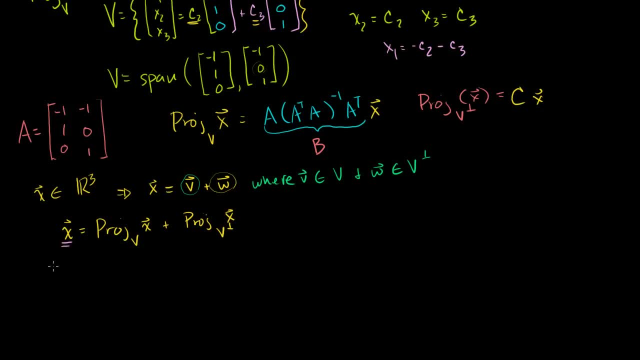 So what are these going to be equal to? Well, x. If I want to write it as a linear transformation of x, I could just write it as the Three by three identity matrix Times: x. Right, That's the same thing as x. 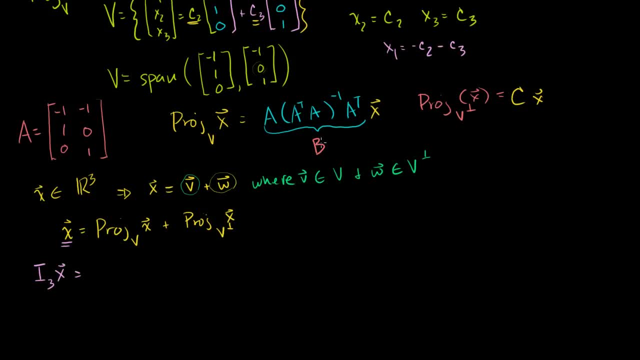 That's going to be equal to the projection of x Onto v. Well, that's just the same thing As b times x. That's the same thing as b Times x, And then plus the projection of x Onto v's orthogonal complement. 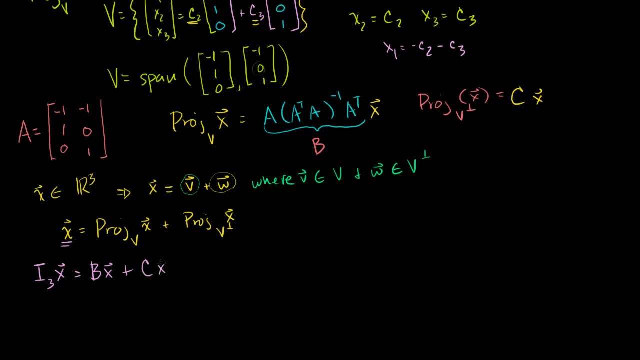 Well, that's just c times x Plus c times x, And if you want to Factor out the x on this side, We know that the matrix vector products Exhibit the distributive property, So we could write that the identity matrix Times x. 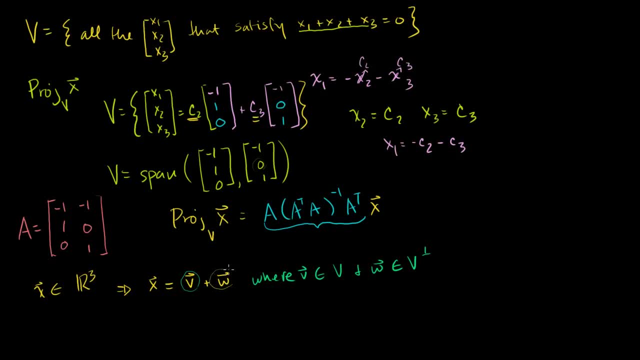 Is the projection of x onto v And this is the projection of x onto the orthogonal complement of v. So we can write that x- x is equal to the projection onto v of x Plus the projection onto v's orthogonal complement Of x. 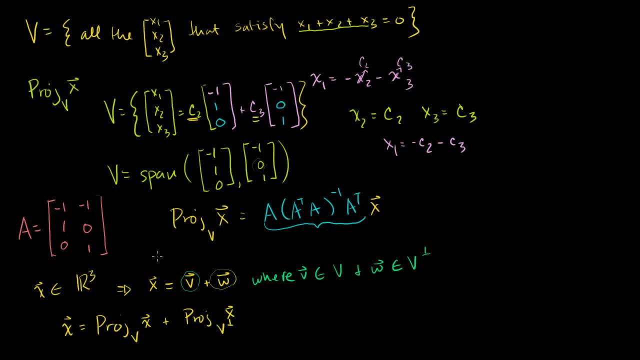 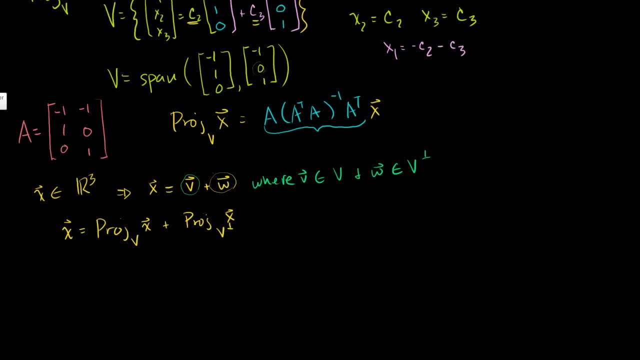 So this is by definition That any member of R3 can be represented this way. Now, if we want to write this as matrix vector products, In two videos ago I showed you that these are linear transformations, So let me write that here. 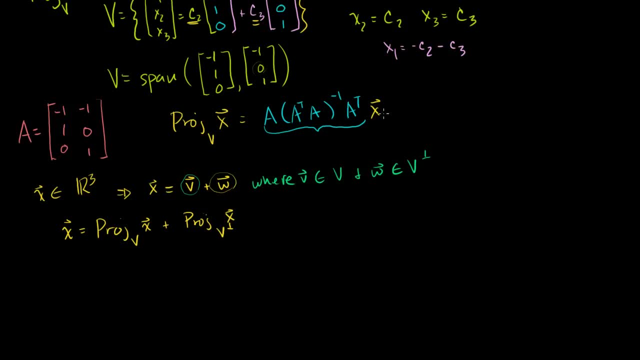 So they're linear transformations, So they can be written as matrix vector products. You see that, right there, Let me define this matrix. I don't know, Let me call this, Let me call this. I don't know, Let's just call this matrix. 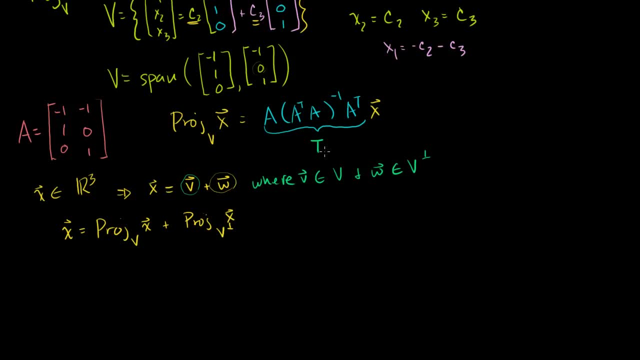 T, T, Let me just call it T And let me call. Let me call, Let me do another, Let me do a letter, Let me do b And let's say that the projection, The projection of Onto the orthogonal complement of v. 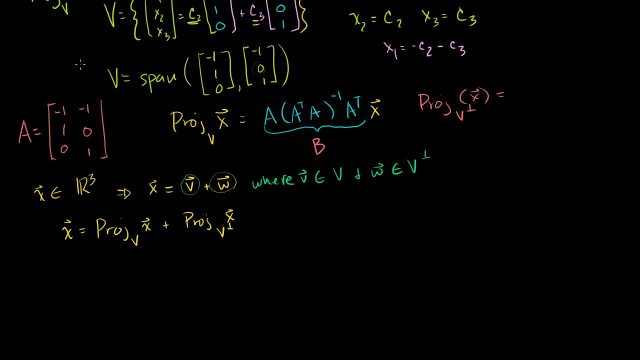 Of x, Let's say that that's equal to some other vector. Sorry, Some other metric, Other matrix C Times x. We know this is a linear transformation, So it can be represented as some matrix C Times x. 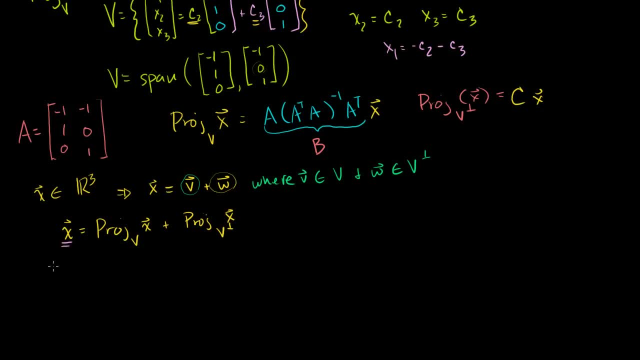 So what are these going to be equal to? Well, x. If I want to write it as a linear transformation of x, I could just write it as the Three by three identity matrix Times: x. Right, That's the same thing as x. 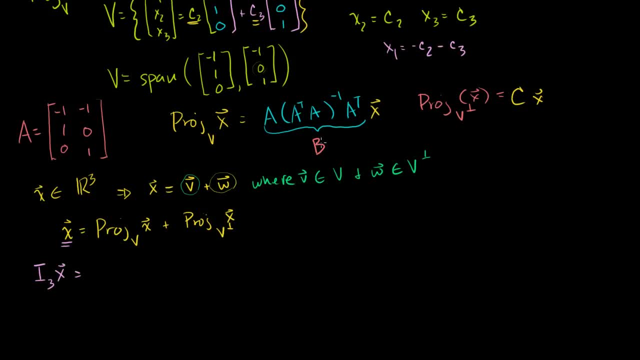 That's going to be equal to the projection of x Onto v. Well, that's just the same thing As b times x. That's the same thing as b Times x, And then plus the projection of x Onto v's orthogonal complement. 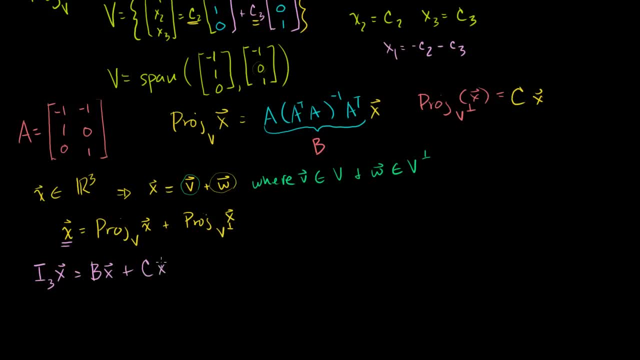 Well, that's just c times x Plus c times x, And if you want to Factor out the x on this side, We know that the matrix vector products Exhibit the distributive property, So we could write that The identity matrix. 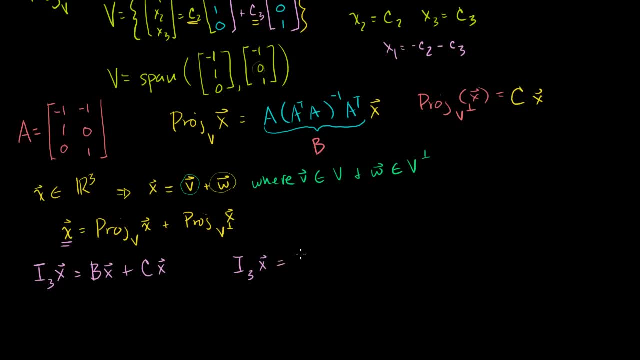 Times x Is equal to B plus c Times x. Or another way to view this equation Is that this matrix Must be equal to These two matrices. So we get that, the identity matrix, The identity matrix In R3.. 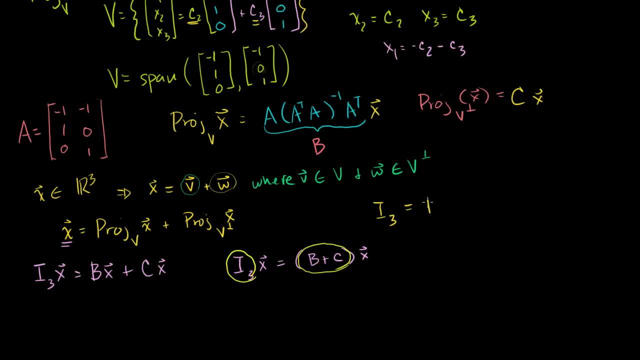 Is equal to The projection matrix onto v Plus the projection matrix Onto V's orthogonal complement. So if we're trying to Remember, the whole point of this problem Is to figure out this thing right here, Is to solve for b. 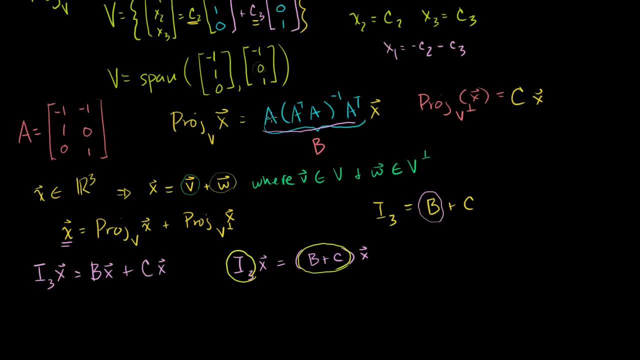 And we know a technique for doing it. You take a transpose. You can do this whole thing, But that might be pretty hairy. But maybe it's easy to find this guy. Maybe, I don't know, It actually turns out in this video. 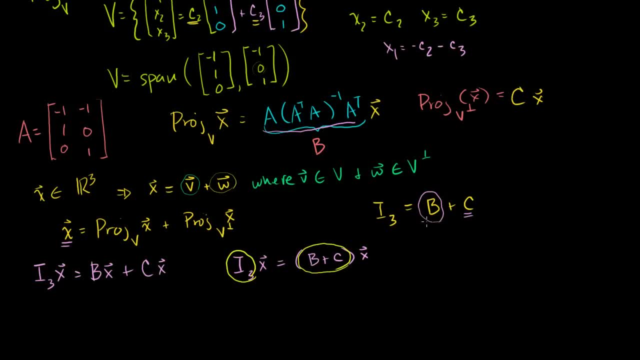 This one will be easy. So if it's easy to find this guy, We can just solve for b. If we subtract c from both sides, We get that b Is equal to, Is equal to, i Is equal to the identity matrix. 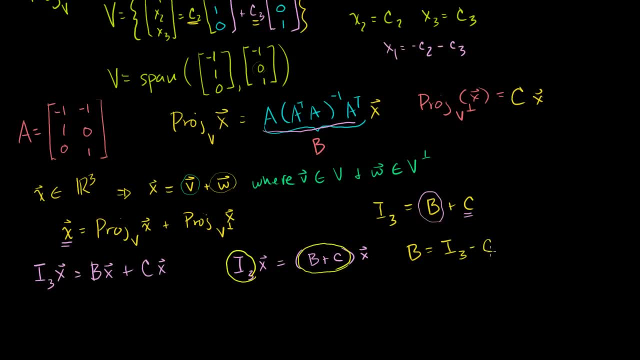 Minus the transformation matrix For the transformation Onto v's orthogonal Complement. So let's see what this is. Let's see if we can figure out What c is Right there. So let's go back to our 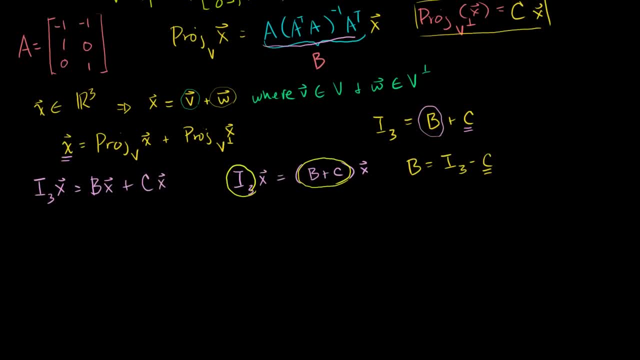 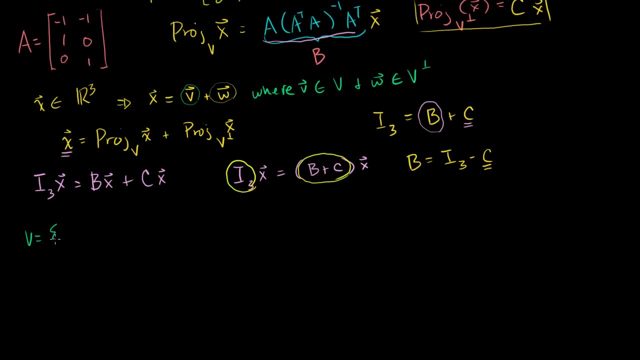 Original. So remember, Let me rewrite the problem, actually Remember that v, Remember that v Was equal to: Essentially Is equal to all of the X1's, X2's, X3's. That satisfies, That satisfy. 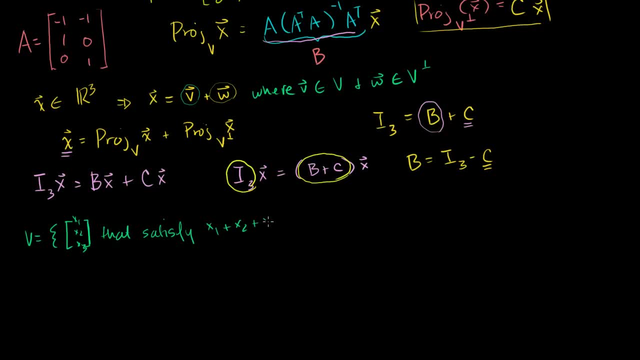 X1. Plus X2. Plus X3. Is equal to zero. Or another way to say, it Is all the X1's, X2's, X3's That satisfy The equation One One. 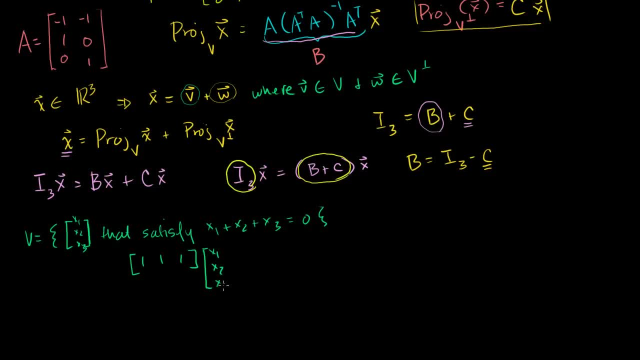 One Times: X1., X2.. X3. Is equal to The zero vector, Or in this case It'll just be zero. We could write the zero vector Like that, Just like that. So one Times. 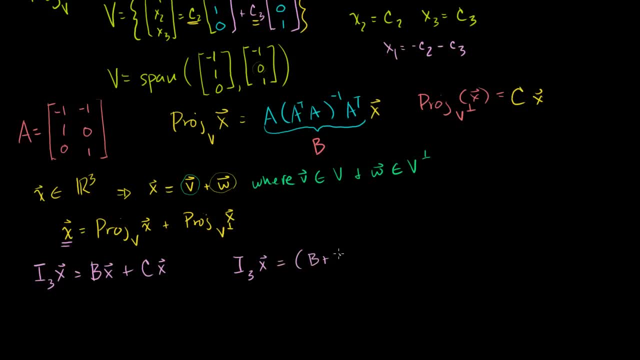 Is equal to B plus c Times x. Or another way to View this equation Is that this matrix Must be equal to These two matrices. So we get that the identity matrix- The identity matrix In R3. Is equal to. 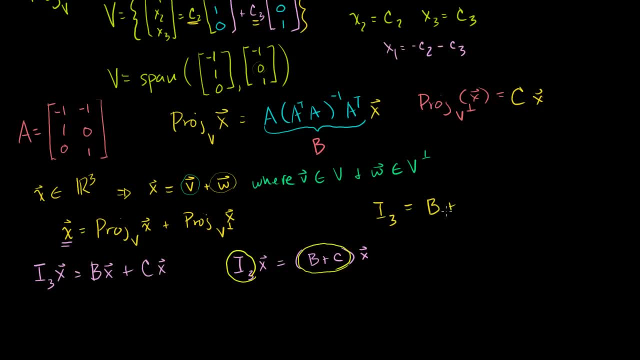 The projection matrix onto v Plus the projection matrix Onto V's orthogonal complement. So if we're trying to Remember, the whole point of this problem Is to figure out this thing right here, Is to solve for b, And we know a technique for doing it. 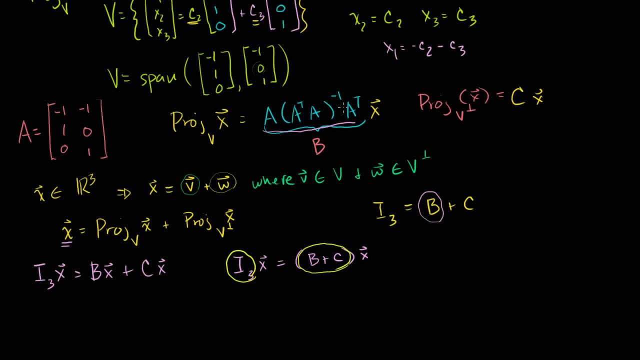 You take a transpo, You do, You can do this whole thing, But that might be pretty hairy. But maybe it's easy to find this guy. Maybe, I don't know, It actually turns out in this video. This one will be easy. 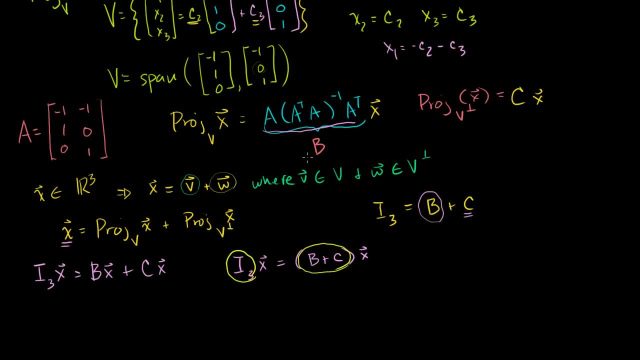 So if it's easy to find this guy, We can just solve for b. If we subtract c from both sides, We get That b Is equal to, Is equal to I, is equal to the identity matrix Minus The transformation matrix. 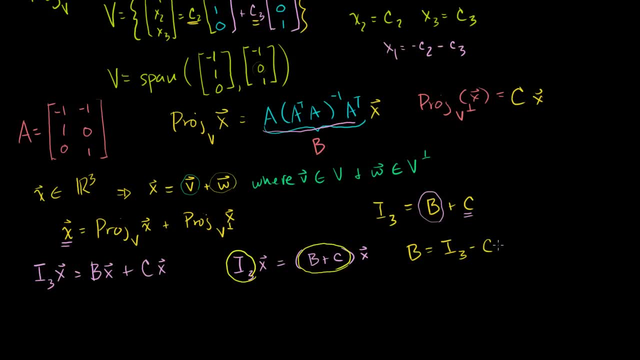 For the transformation Onto v's orthogonal Complement. So let's see what this is, Let's see if we can figure out What c is Right there. So let's go back to our Original. So remember, Let me rewrite. 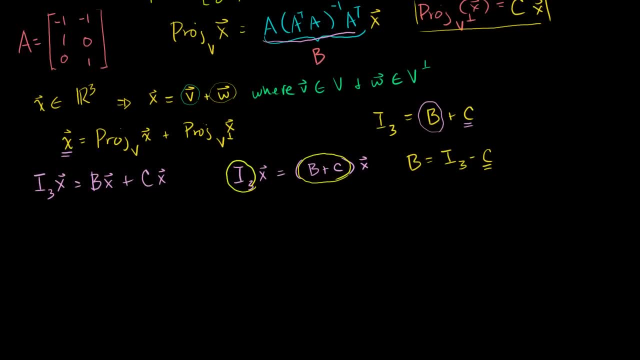 The problem. actually, Remember that v, Remember that v Was equal to Essentially Is equal to all of the X1's, X2's, X3's. That satisfies, That satisfy X1. Plus X2.. 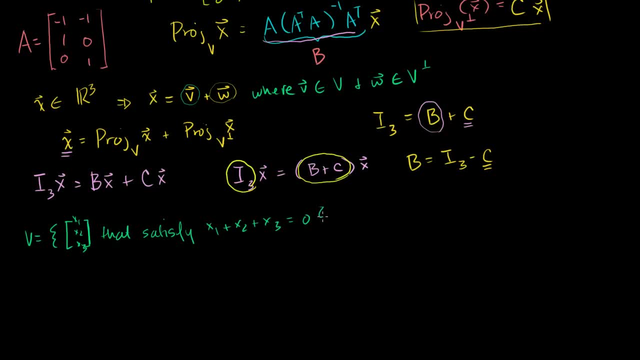 Plus X3. Is equal to 0. Or another way to say: it Is all the X1's, X2's, X3's That satisfy The equation 1.. 1. 1. Times. 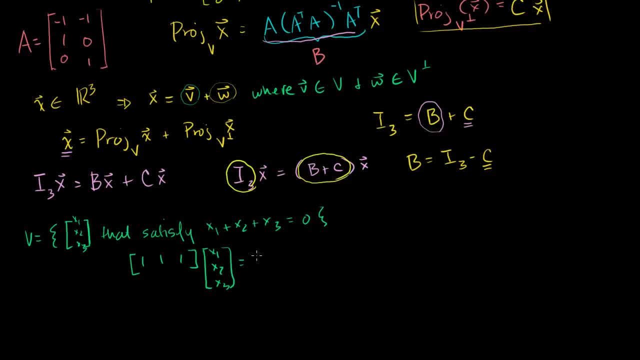 X1. X2.. X3. Is equal to The 0 vector, Or in this case It'll just be 0. We could write the 0 vector Like that, So: 1. Times X1. Plus. 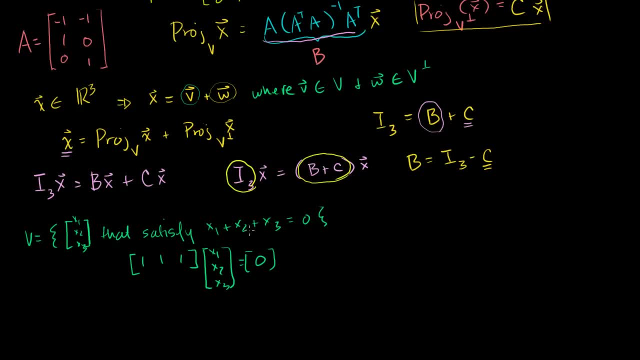 X1. Plus One Times X2. Plus One Times X3. Is going to equal the zero vector. This is another way to write v. Now All of the x's that satisfy this right here. What is that? 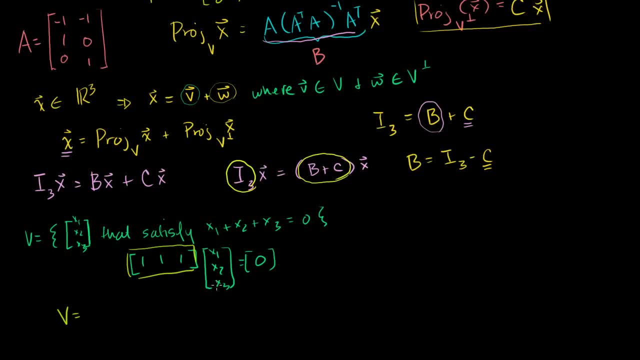 This. This is saying that v is equal to the null space Of This Matrix. Right there, Right, The null space of this matrix Is all of the vectors that satisfy this equation. So v Is equal to The null space. 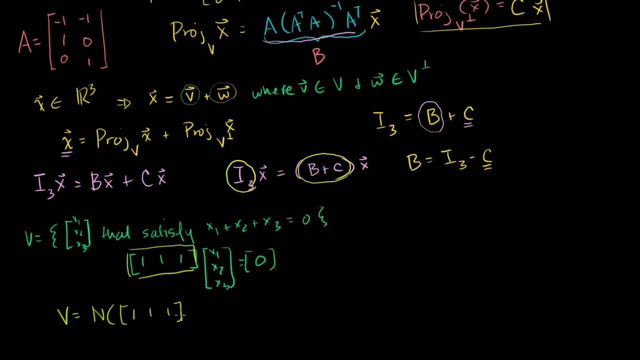 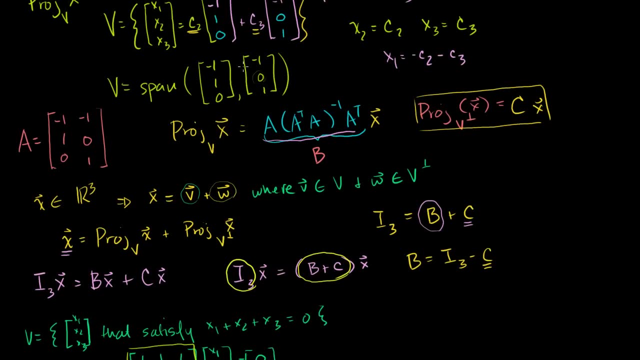 The null space Of One One One, Just like that. Up here We kind of Figured out v In kind of the traditional way. We figured out that v Is the span of these things. But now we know, 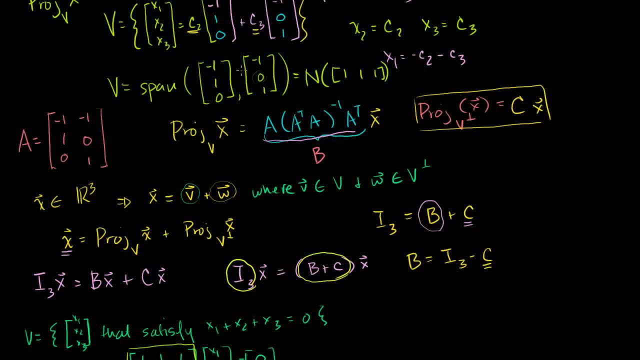 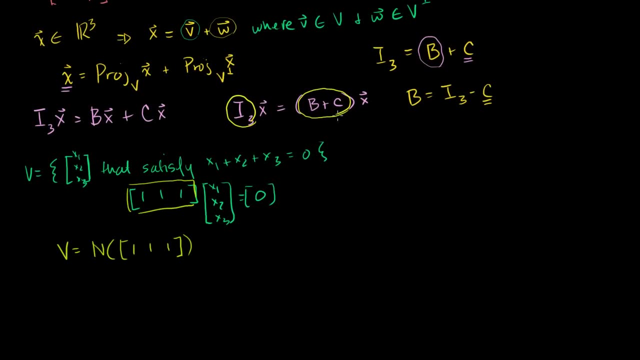 That's the same thing as the null space Of One One One. These two statements are equivalent. Now We, At least At a hunch That maybe You know, We could figure out Straight up The. 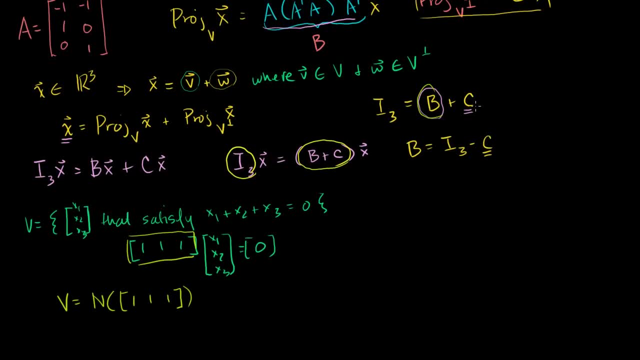 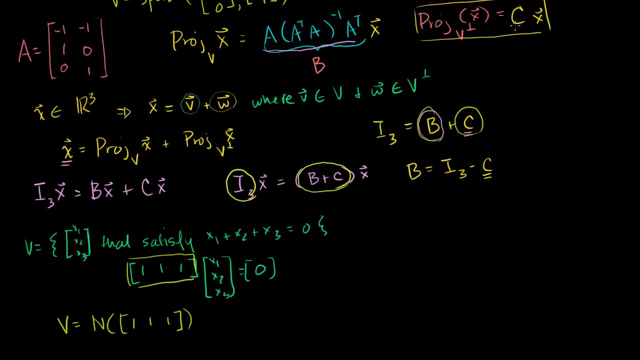 This b here. By doing all of this- A transpose, We can figure out The Transformation Matrix For The orthogonal complement Of v, For the orthogonal complement Of v, Right there. But then we can just apply. 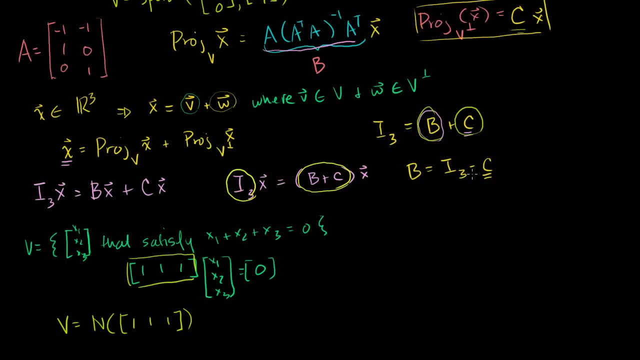 This kind of That we can just solve for b, Given that The identity matrix Minus This guy Is going to be equal to b. So let's see if we can figure out. Let's see if we can figure out. 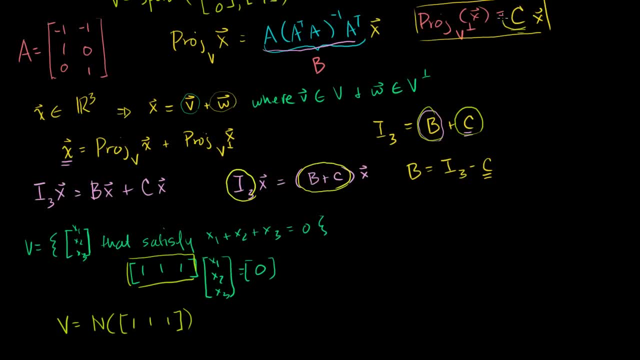 The projection matrix, If we can figure out The, The transformation matrix For the orthogonal projection For x Onto the orthogonal projection Of v. So this, This is v. What is What is V complement, V, complement. 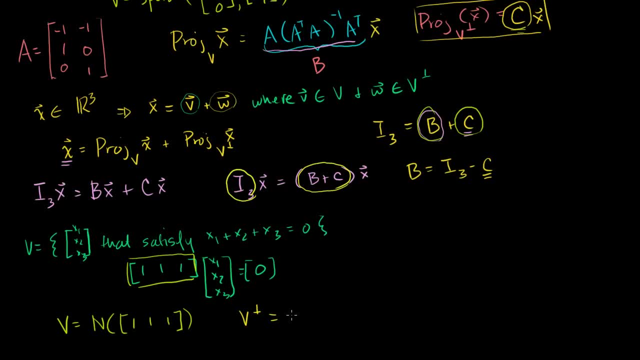 Is going to be equal to The Orthogonal complement, Or v perp Is going to be equal to The orthogonal complement Of the null space Of this, Of this Matrix Right here, Which is equal to what? 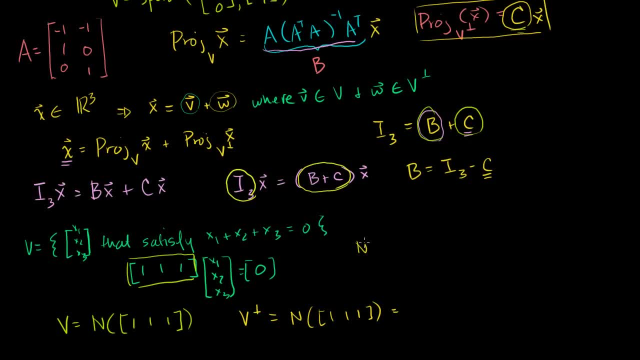 Remember The null space? It's Orthogonal complement, The A null space's Orthogonal complement Is Equivalent To The Rowspace Or the column space Of A Transpose. We saw that. 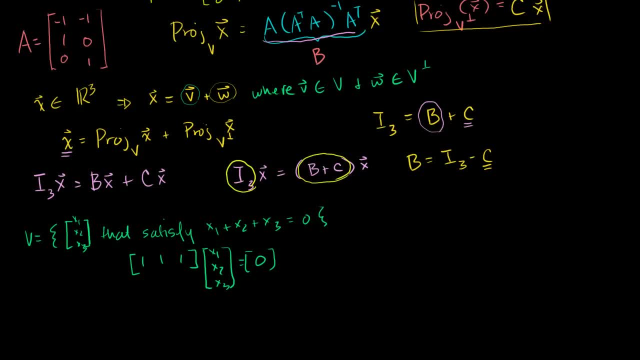 1. Times X2. Plus 1. Times X3. Is going to equal the 0 vector. This is another way to write v. Now All of the x's that satisfy this right here. What is that? 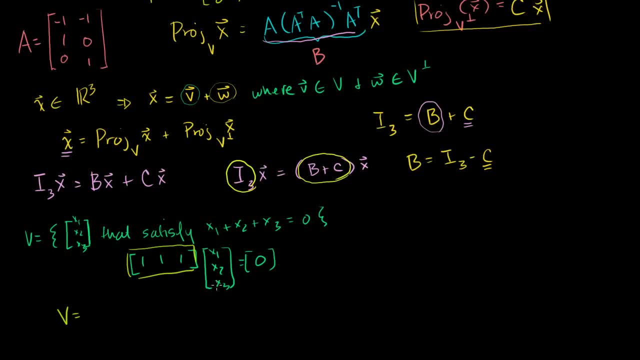 This. This is saying that v is equal to the null space Of This Matrix. Right there, Right, The null space of this matrix Is all of the vectors that satisfy this equation. So v Is equal to The null space. 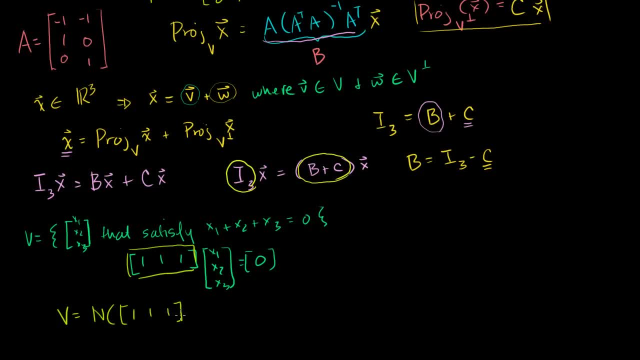 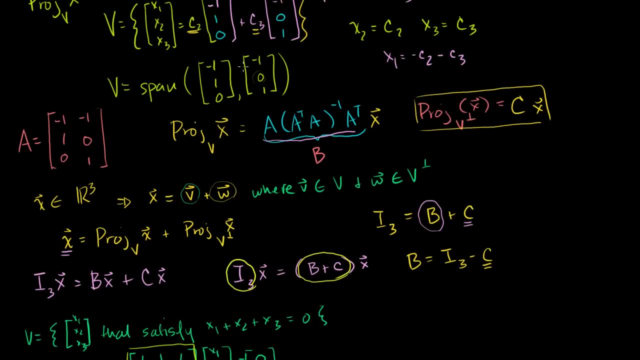 The null space Of 1.. 1.. 1. Just like that. Up here We kind of Figured out v In the kind of the traditional way. We figured out that v Is the span of these things. 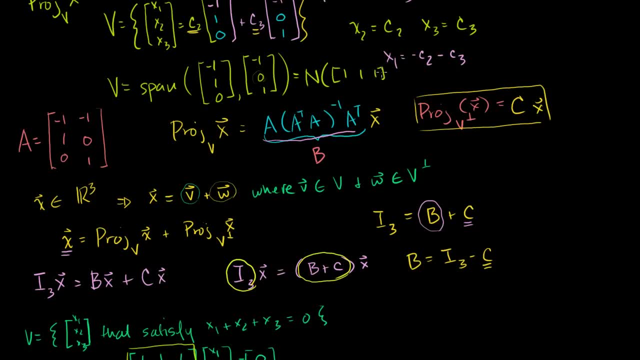 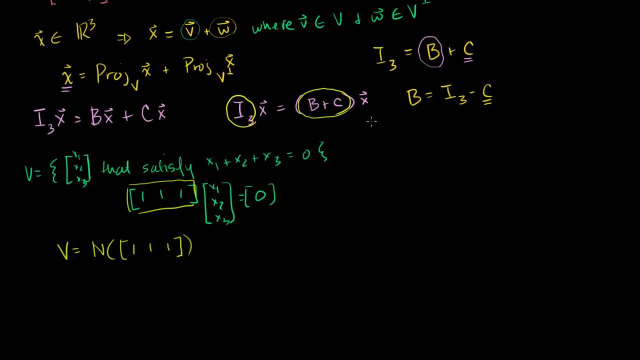 But now we know That's the same thing as the null space Of 1. 1. 1. These two statements are equivalent. Now We, At least At a hunch, That maybe You know We could figure out. 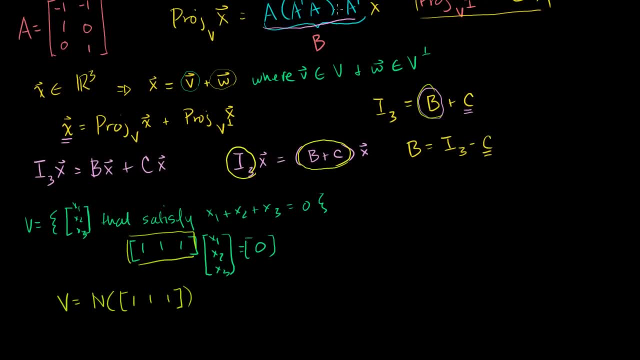 Straight up The This b here By doing all of this. So the hunch is: Maybe if we can figure out The Transformation Matrix For The orthogonal complement Of v. For the orthogonal complement Of v. 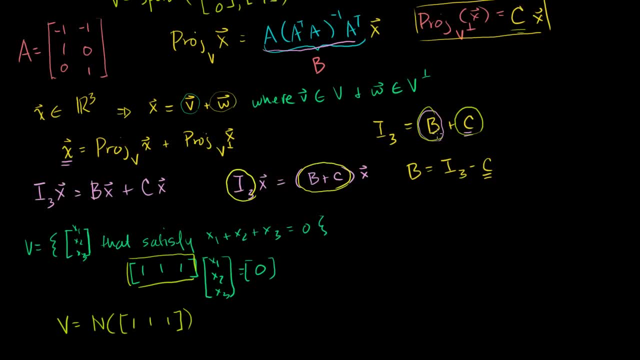 Right there. Then we can just apply This kind of That. we can just solve For b. Given that The identity matrix Minus This guy Is going to be Equal to b. So let's see if we can figure out. 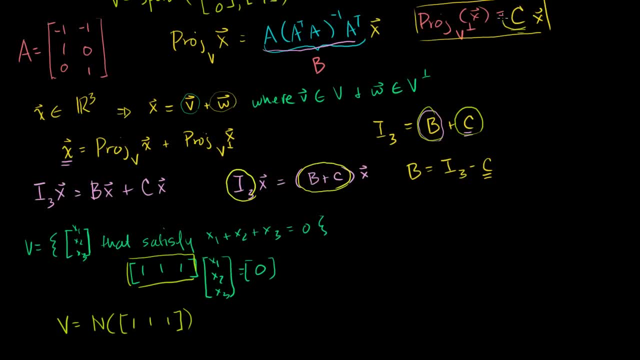 Let's see if we can figure out The projection matrix, If we can figure out The, The transformation matrix For the orthogonal projection For x Of v. So this, This is V. What is? What is V complement? 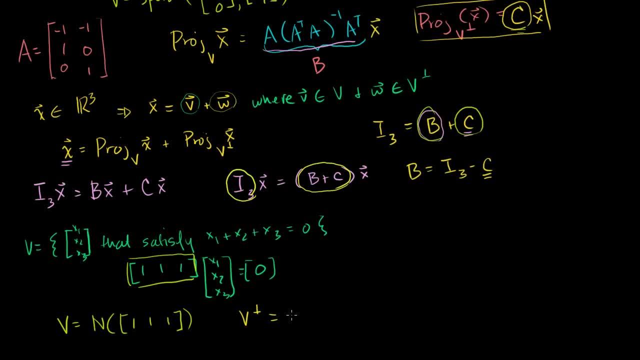 V Complement Is going to be Equal to The Orthogonal complement, Or v perp Is going to be Equal to The orthogonal complement Of the null space Of this, Of this Matrix Right here. 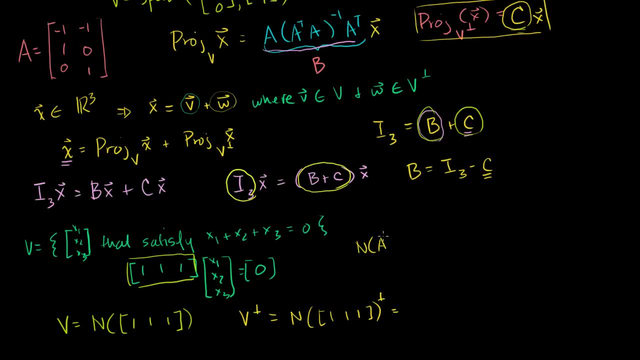 Which is Equal to what Remember The null space. It's Orthogonal complement. The Transpose Is Equivalent To Is Equivalent To The row space Or the column space Of a Transpose. 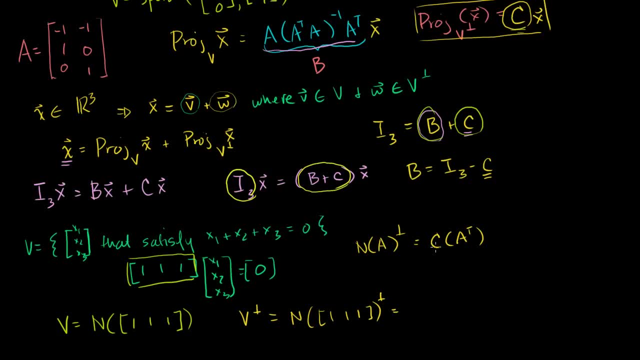 Multiple times. Or you could say The, The. The Orthogonal complement Of The rowspace Is The null space. We've seen this Many, many times before. So The Orthogonal complement Of This guy. 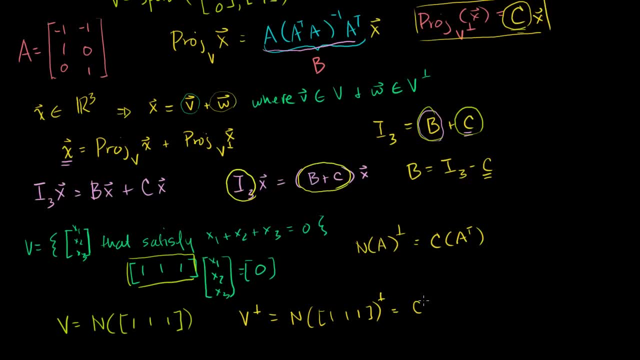 Is going to be the column space Of his transpose, So the column space Of the transpose Of this guy. So It's One One, One, Just like that. Or We can write, Or We can write. 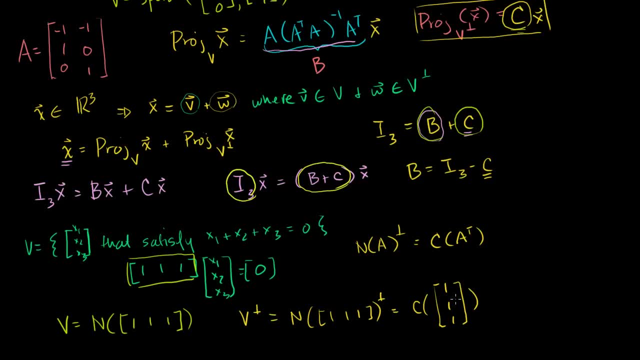 That V, V's Orthogonal complement Is equal to The span, The span Of One One, One Right, The column space Of this matrix. We only have One column in it, So It's column space. 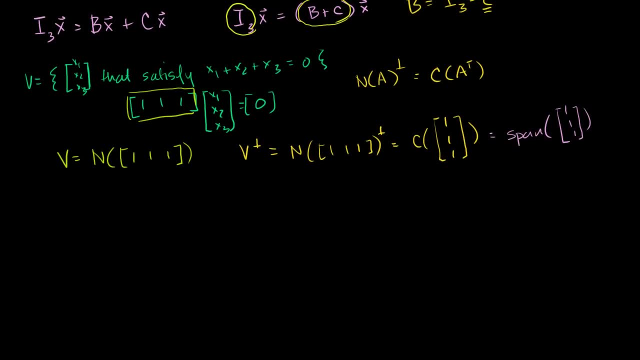 Is going to be the span Of that one column. So The original Equation For V That satisfies that That's just going to be some plane In R3.. That's going to be some plane In R3.. 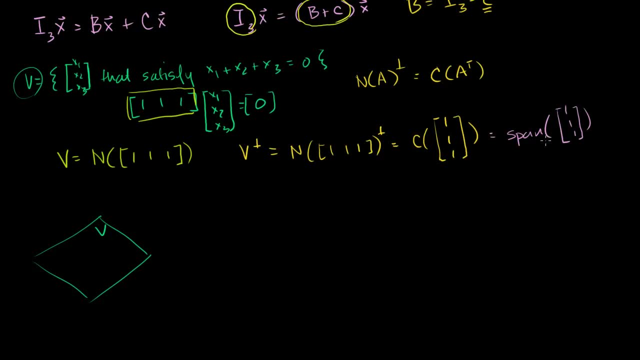 That is V, Right there. And now We just figured out what V's Orthogonal complement Is. It's going to be a line In R3.. Right, It's going to be all of the linear combinations Of this guy. 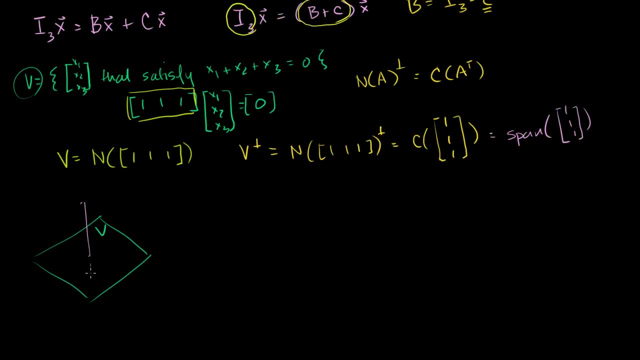 So It's going to be some line In R3.. I haven't drawn it. You know This is going to be tilted more And so is this, But it's going to be some line. So Remember The projection. 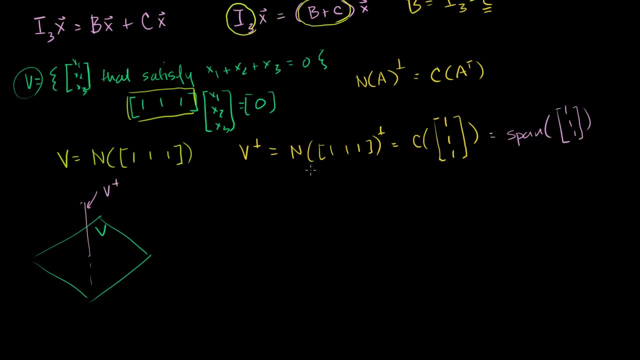 The projection. Let me do it this way. So Let's create. So This is the basis For V's orthogonal complement. So Let's construct Some matrix. Let's construct Some matrix, I don't know. 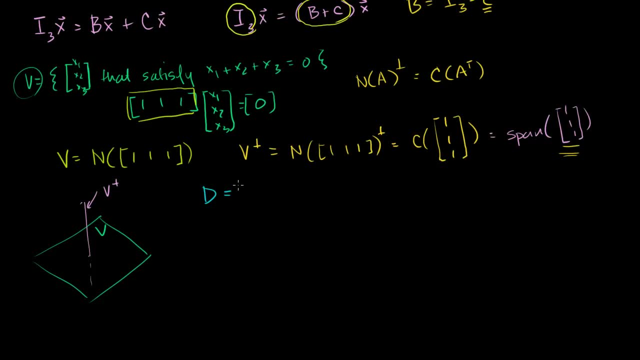 Let me use a new letter That I haven't used before. Let me construct Some matrix D Whose columns Are the basis vectors For the orthogonal complement Of V? Well, There's only one basis vector, So 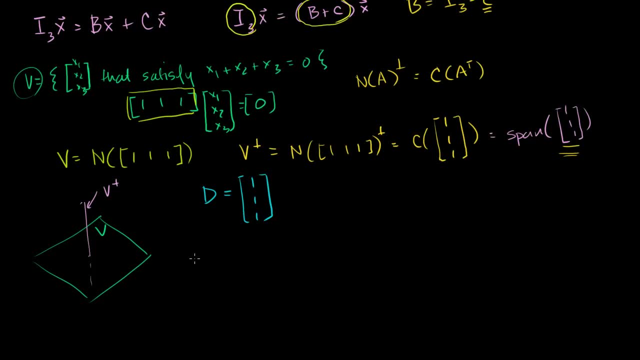 It's going to be that. So It's going to be that, And we learned The last video And the video before that That the projection, The projection Of Any vector In R3.. Onto V's. 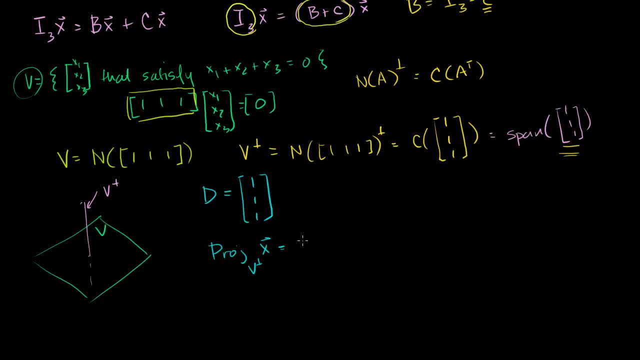 Orthogonal complement Is going to be equal to: D Times D Transpose D. Inverse Times D Transpose Times D Transpose Times D Transpose Times X, Or another way to view it. 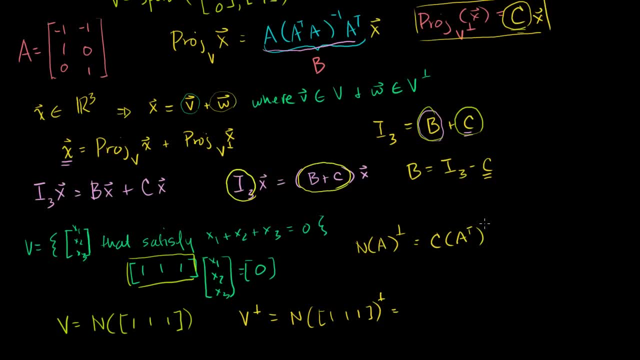 We saw that Multiple times. Or you could say The, The, The Orthogonal complement Of The row space Is The null space. We've seen this Many, many times before. So The Orthogonal complement. 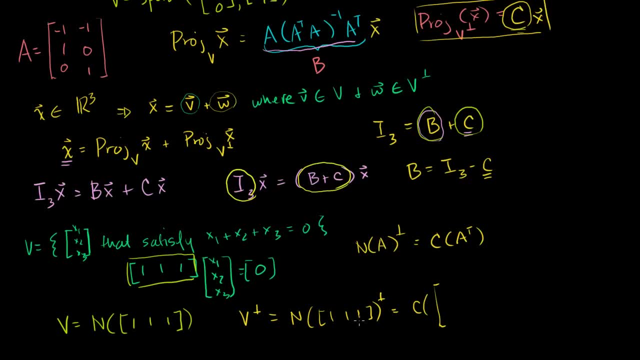 Of This guy, Of The Transpose Of This guy, Right? So It's One, One, One, Just like that. Or We can write, Or We can write That V V's. 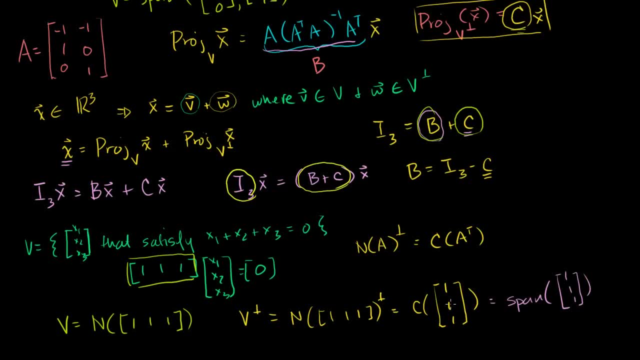 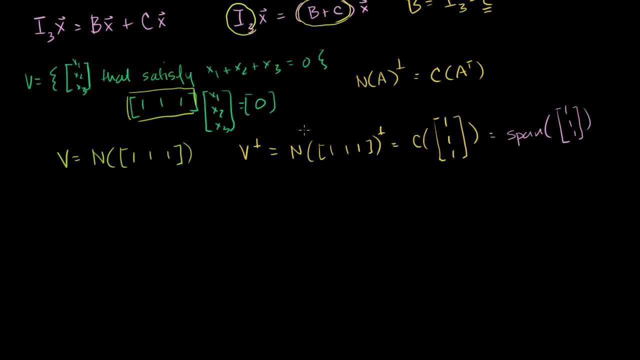 Orthogonal complement Is Equal to The span, The span Of One One, One Right. So What we're doing here, That Original Equation For V That Satisfies That. 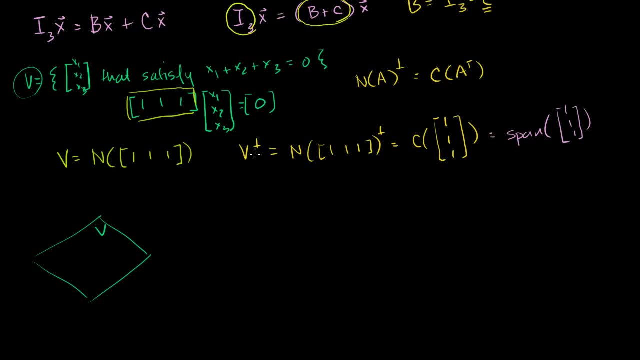 That's just going to be some plane in R3.. That's going to be some plane in R3.. That is V Right there, And now We just figured out what V's Orthogonal complement Is. It's going to be a line in R3.. 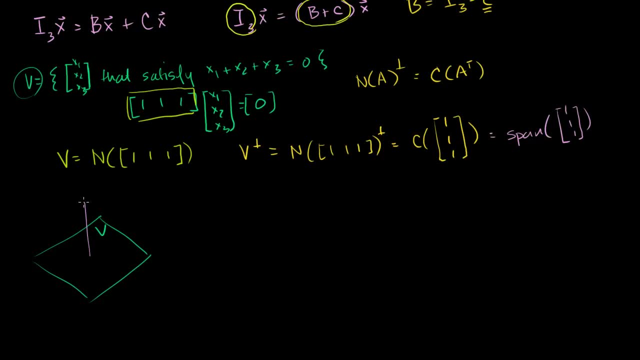 Right, It's going to be all of the linear combinations Of This guy, So It's going to be some line in R3.. I haven't drawn it. You know This is going to be tilted more, And so is this. 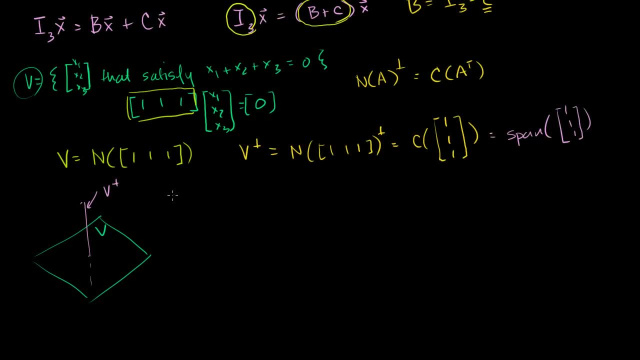 So let's see if we can Figure out. So remember, The projection, The projection. Let me do it this way. So let's create. So this is The basis For V's orthogonal complement. So let's construct. 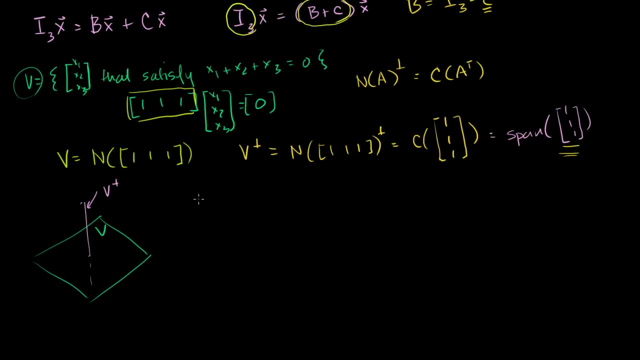 Some Matrix. Let's construct Some matrix. I don't know. Let me use a new letter That I haven't used before. Let me construct Some matrix D, Whose columns Are the basis vectors For the orthogonal complement. 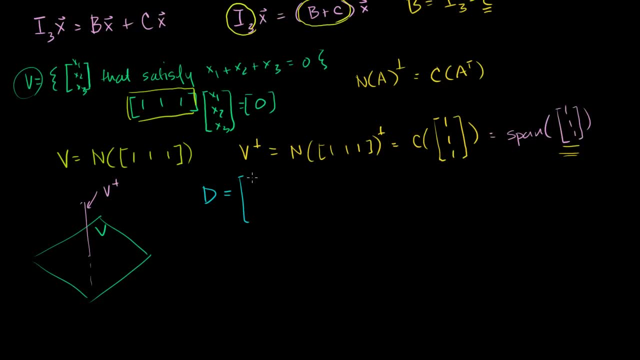 Of V. Well, There's only one basis vector, So It's going to be that And We learned The last video And the video before that That the projection, The projection Of Any vector In R3.. 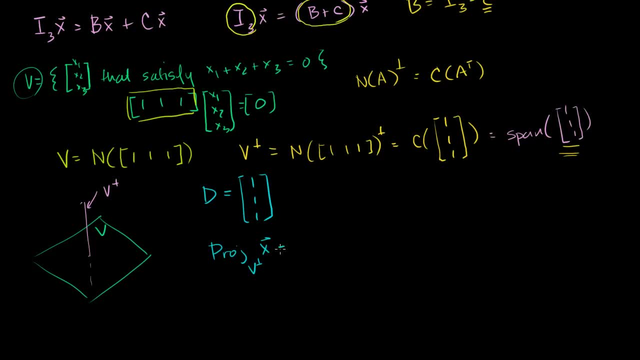 Onto, V's Orthogonal complement Is going to be equal to: D. Times D Transpose D. Inverse Times D Transpose Times D Transpose Times X Or. 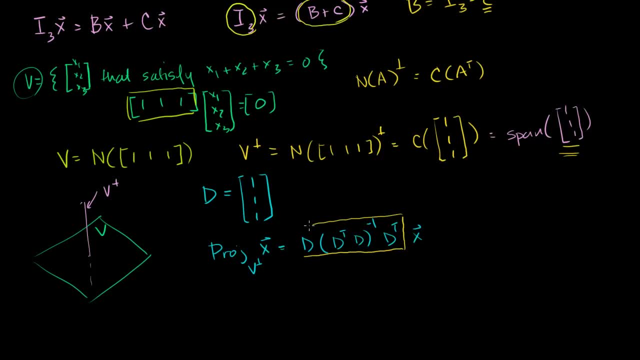 Where, Or I can just use A single matrix. It's going to be this. So How Is it? You can, You can. You can do this, You can do this. It's going to work So. 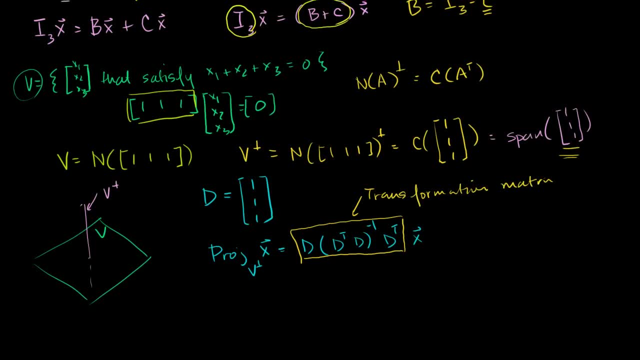 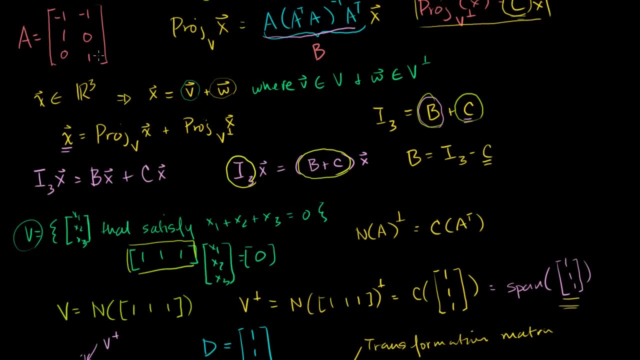 What you have to do Is that This Thing right Here, That thing right there, Is The transformation matrix For this Projection. That is the Transformation matrix, Transformation Matrix, So I2 matrix. it seems pretty difficult. 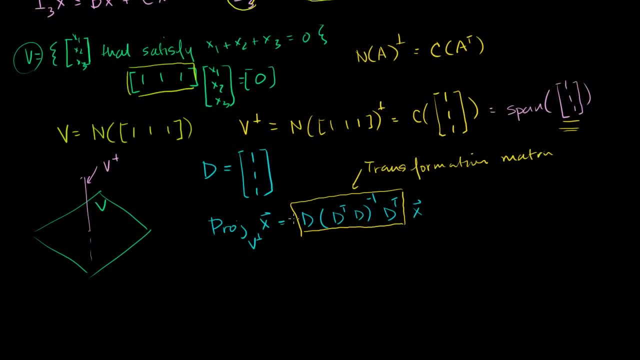 Instead, let's find the projection matrix to get to the projection onto v's orthogonal complement, which is this: So what is d transpose? So d transpose is just going to be equal to 1, 1, 1.. What is d transpose times d? 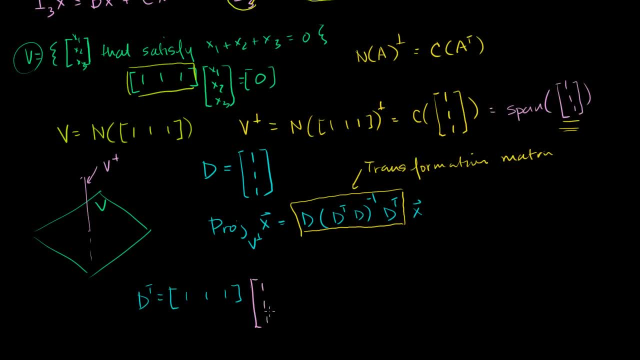 Well, that's d transpose. This is d, just like that. So what is this going to be equal to? This is just the dot product of that and that right. 1 times 1 plus 1 times 1 plus 1 times 1, it equals 3.. 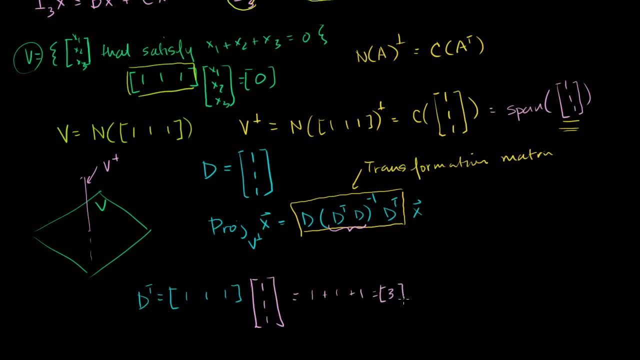 So this thing right here is equal to a 1 by 1 matrix 3.. So let's write down: So this is equal to d, which is this matrix 1, 1, 1, times d. transpose d inverse. 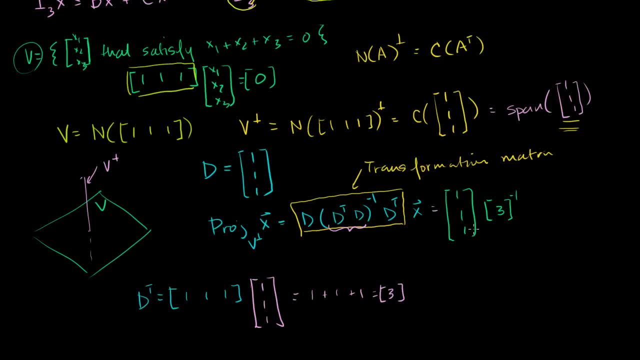 So d transpose d is just a 1 by 1 matrix. We're going to have to invert it. Actually, I've never defined the inverse of a 1 by 1 matrix. I gave you the matrix for you just now. so this is mildly. 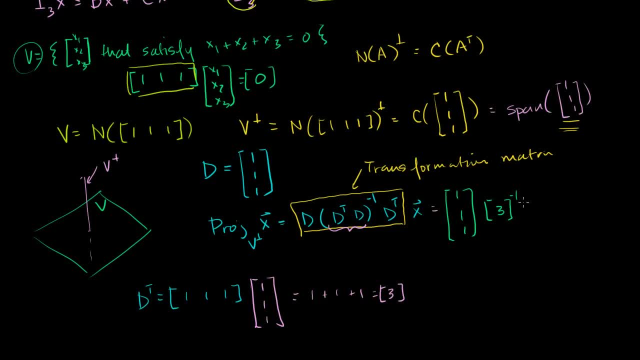 exciting times: d transpose. So d transpose looks like this: 1,, 1,, 1.. And then all of that's times x, But this is the transformation matrix, right there. Now, what is the inverse of a 1 by 1 matrix? 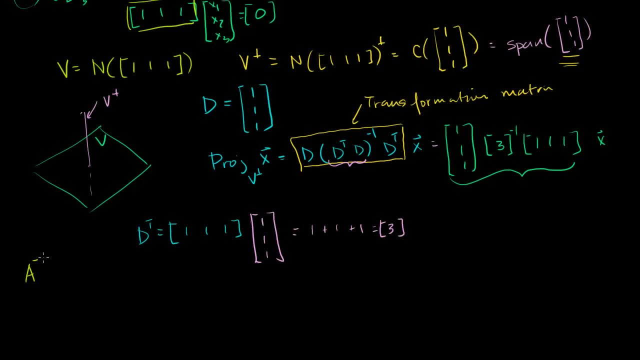 Now you just have to remember that a inverse times a is equal to the identity matrix. If we're dealing with a 1 by 1 matrix, then I'm just trying to figure out what, Let's say what matrix times 3 is going to be equal to the 1. 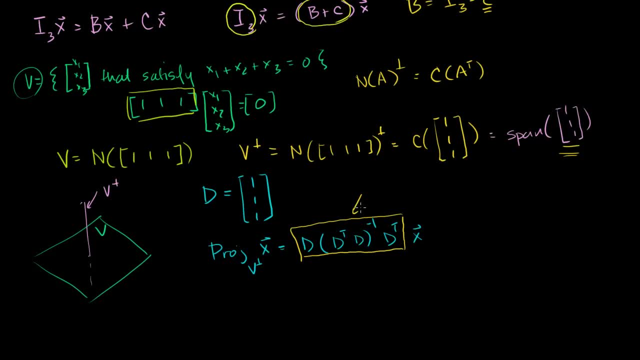 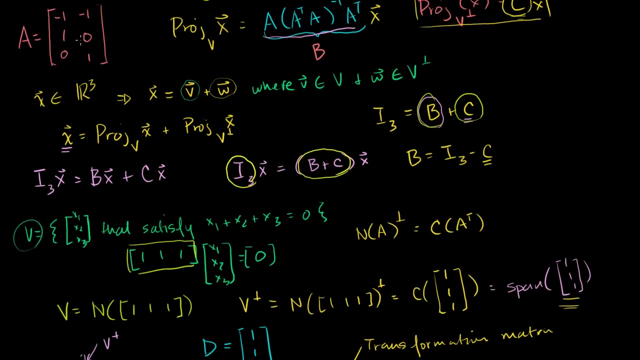 That thing. right, there Is the transformation matrix For this projection. That is the transformation matrix, Transformation Matrix. So let's see if this is easier to solve This thing Than This business up here Where we had a 3 by 2 matrix. 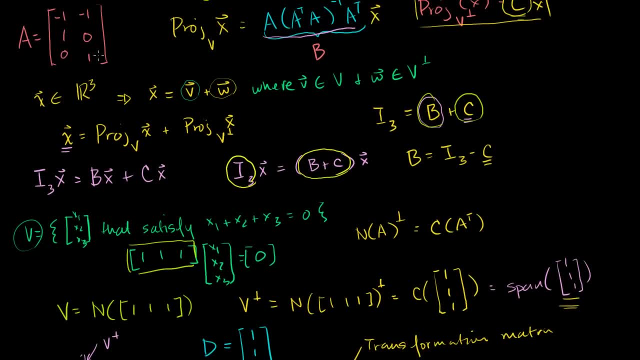 That was the whole motivation For doing this problem: To figure out the projection matrix For V subspace. We'd have to do this With the 3 by 2 matrix. It seems pretty difficult. Instead, Let's find the projection matrix. 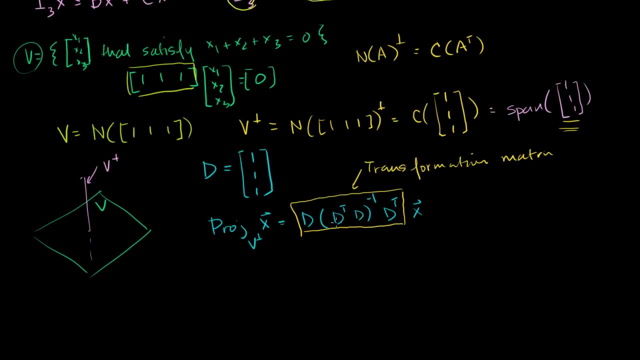 To get to The projection Onto V's orthogonal complement, Which is this: So what is D transpose? So D transpose Is just going to be equal to 1, 1, 1.. What is D transpose times D? 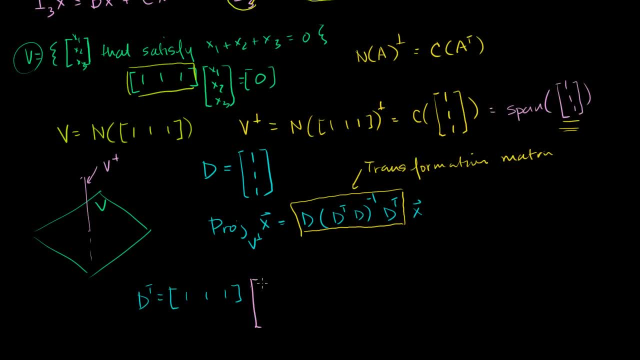 Well, That's D transpose. This is D, Just like that. So what is this going to be equal to? This is just the dot product Of that and that Right 1 times 1.. Plus 1 times 1.. 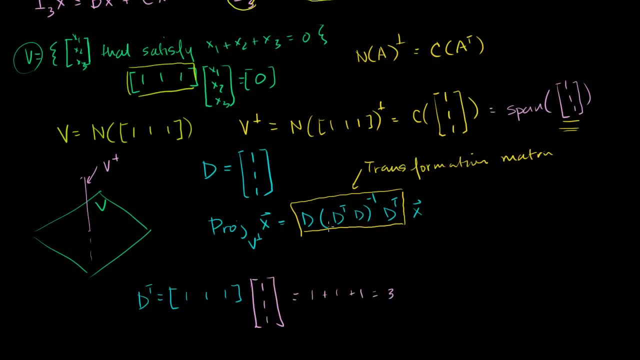 Plus 1 times 1. It equals 3.. So this thing right here Is equal to a 1 by 1 matrix 3.. So let's write down: So this is equal to D, D, Which is this matrix? 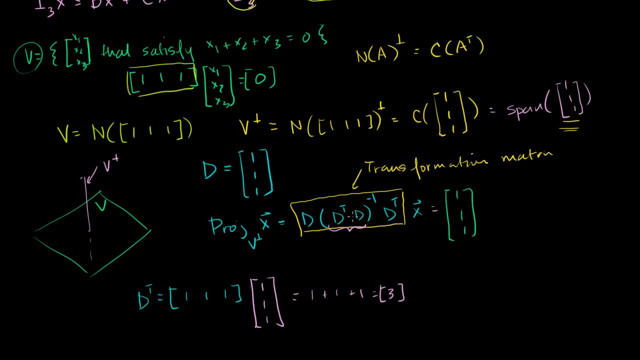 1, 1, 1. Times D transpose D inverse. So D transpose D Is just a 1 by 1 matrix. We're going to have to invert it. Actually, I've never defined The inverse of a 1 by 1 matrix. 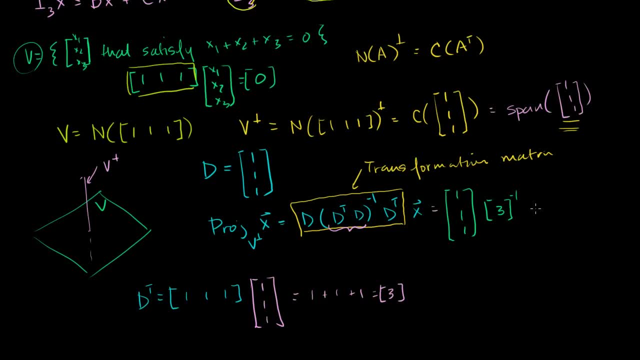 For you just now. So this is mildly exciting. Times D transpose. So D transpose Looks like this: 1, 1, 1.. And then all of that Times X. But this is the transformation matrix, Right there. 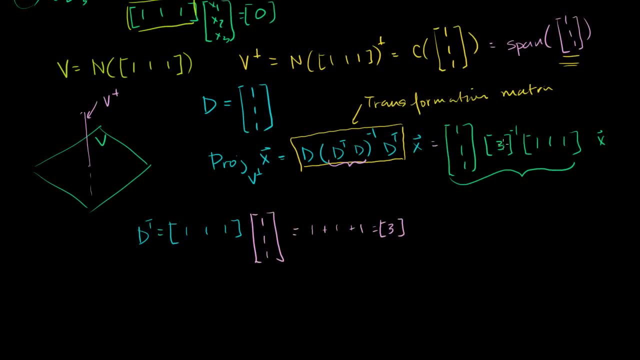 Now, What is The inverse of a 1 by 1 matrix? Now you just have to remember, You just have to remember That A inverse Times A Is equal to the identity matrix. If we're dealing with a 1 by 1 matrix. 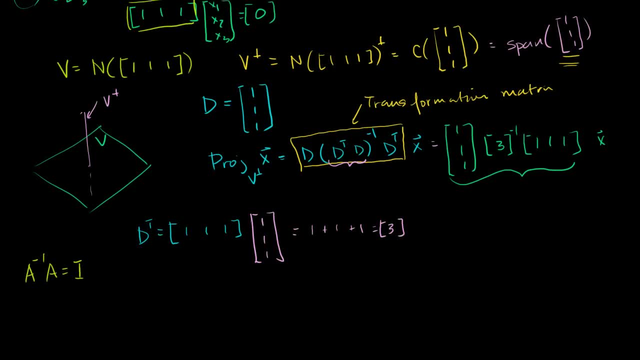 Then we're just- I'm just trying to figure out What- Let's say What- matrix Times 3. D, D, D, D, D D D. Times 3. Is going to be equal to the 1 by 1 identity matrix. 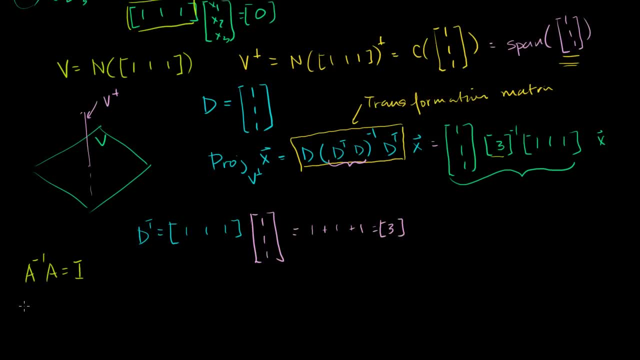 by 1 identity matrix. So if I say, let's say, you know, I don't know, let's say that 3 inverse times 3 has to be equal to the identity matrix 1 by 1 identity matrix, Well, the only matrix that's going to make this work out. 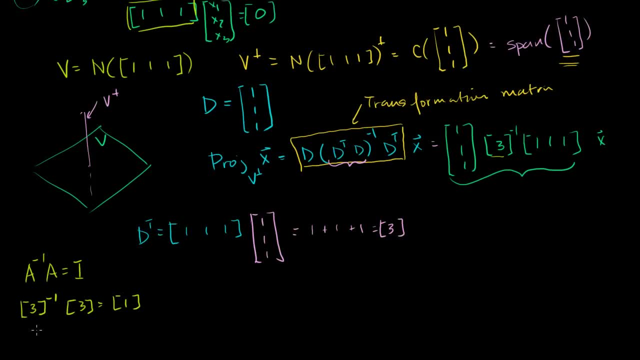 to get this entry I have to take this guy's entry. times that guy's entry. It's going to be this guy right here. The inverse of this 1 by 1 matrix has to be the matrix 1 third. 1 third times 3 is equal to 1.. 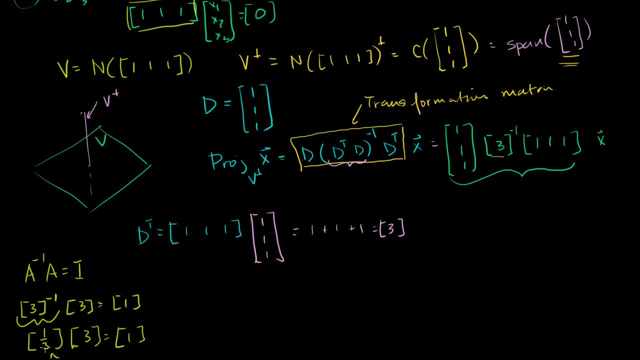 This is almost trivially simple, but this is the inverse. that right there is the inverse matrix for the 1 by 1 matrix 3.. So this right here is just 1 third, And we could actually just take that out. It's a 1 by 1 matrix, which is essentially 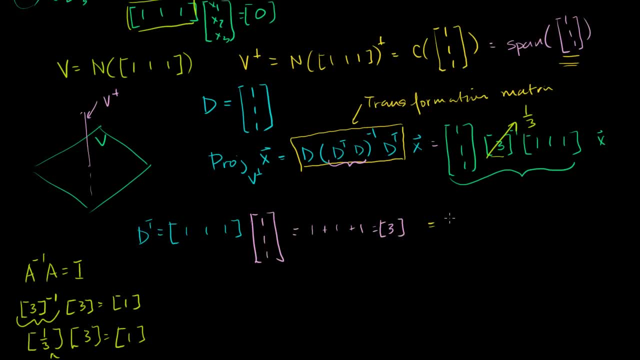 equivalent to a scalar. So this is going to be equal to. Let me just draw a line here: This thing is equal to 1 third. Actually, I don't want to confuse you, Let me rewrite it So we get the projection of any vector in R3 onto the. 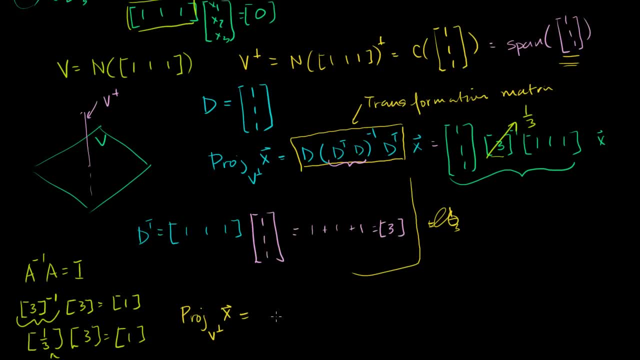 orthogonal complement of V is equal to 1 third times the vector 1, 1, 1 times sorry, oh yeah, it is a vector, or the matrix 1 on 1.. Times that matrix. Transition, Transition, Transition. 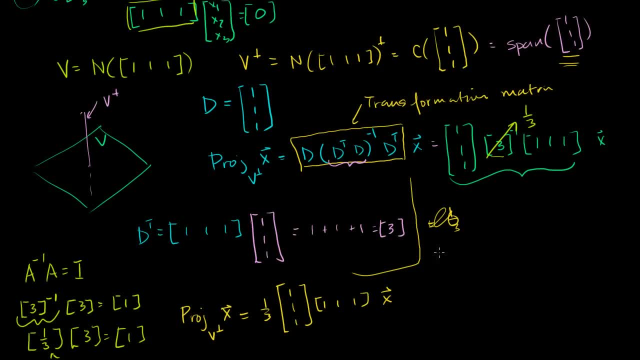 Transpose 1,, 1,, 1.. And then all of that times x, And you can see this is a lot simpler than when we did it with. if we had to do all of this business, if we did all. 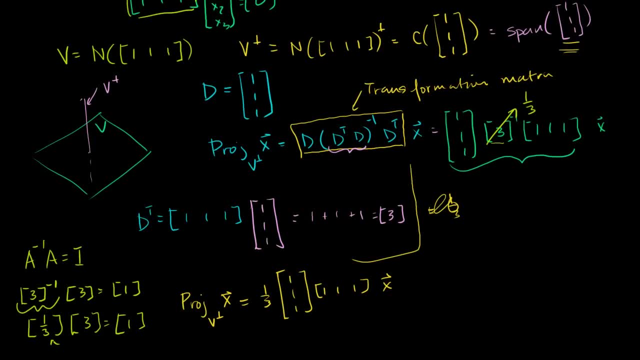 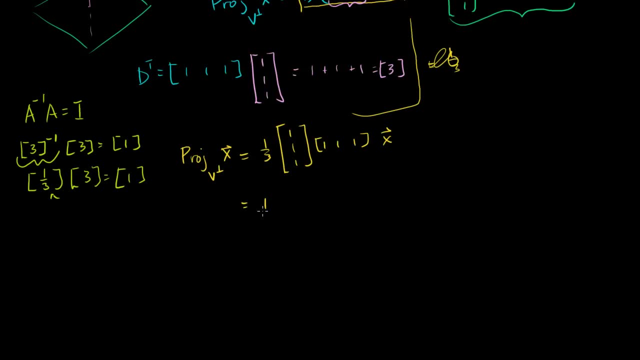 of this business with this matrix. That's a harder matrix to deal with. This 1, 1, 1 matrix is very easy. Now what is this going to be equal to? This is going to be equal to 1 third times. 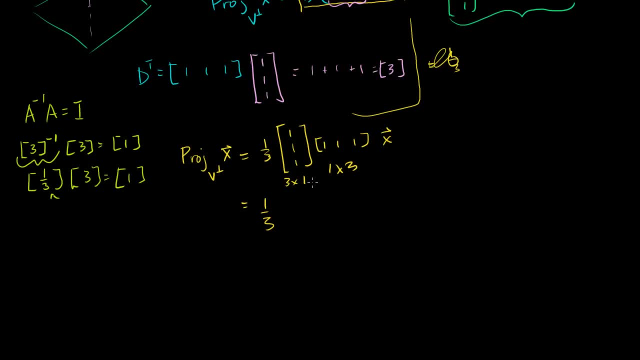 We have a 3 by 1 times a 1 by 3 matrix, so it's going to result in a 3 by 3 matrix, 3 by 3 matrix. And what do we get? The first entry is going to be 1 times 1,, which is 1.. 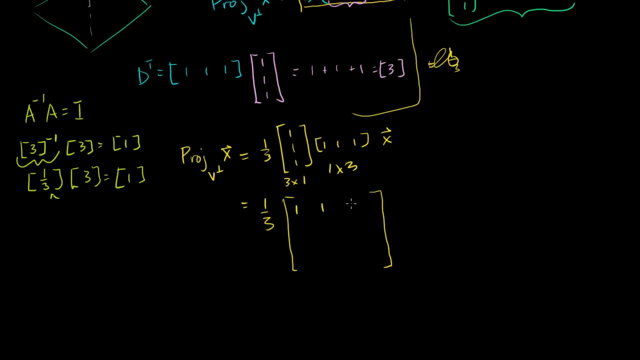 Second entry is going to be 1 times 1,, which is 1.. Third entry is going to be 1 times 1, which is 1.. I think you see the pattern. This guy, the second row, first column, 1 times 1 is 1.. 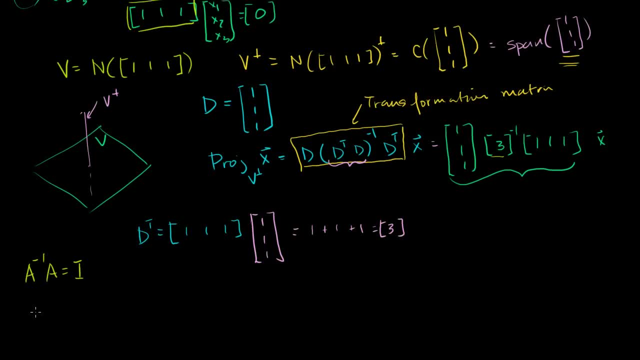 So If I say, Let's say You know, I don't know, Let's say that 3 Inverse 3. Inverse Times, 3. Has to be equal to. Has to be equal to. 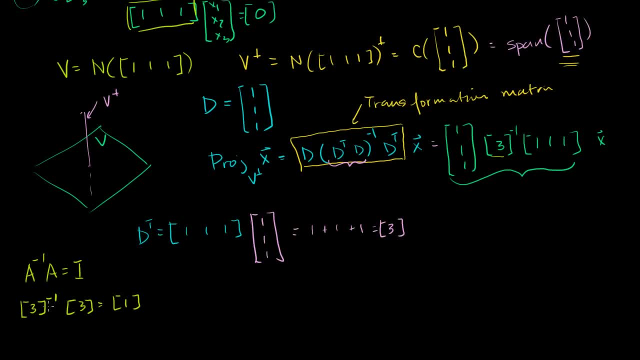 The identity matrix 1 by 1 identity matrix- Well, The only matrix That's going to make this work out. To get this into Have to take This guy's entry Time's. that guy's entry Is going to be this guy. 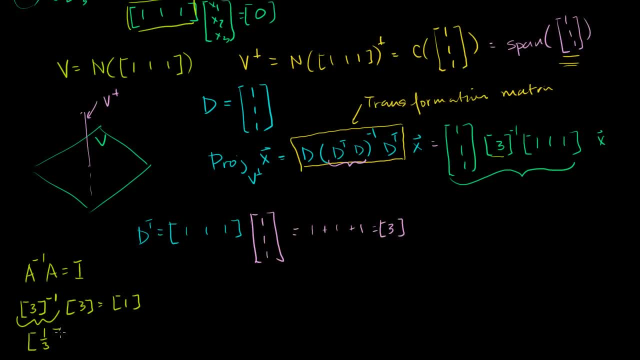 Right by 1 matrix has to be the matrix 1 third. 1 third times 3 is equal to 1.. This is almost trivially simple. but that right there is the inverse matrix for the 1 by 1 matrix 3.. 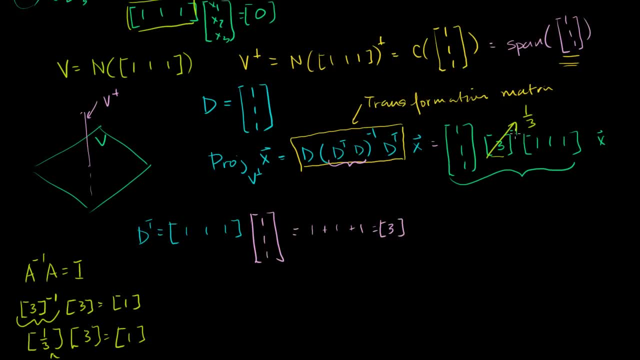 So this right here is just 1 third, And we could actually just take that out. It's a 1 by 1 matrix, which is essentially equivalent to a scalar. So this is going to be equal to. let me just draw a line. 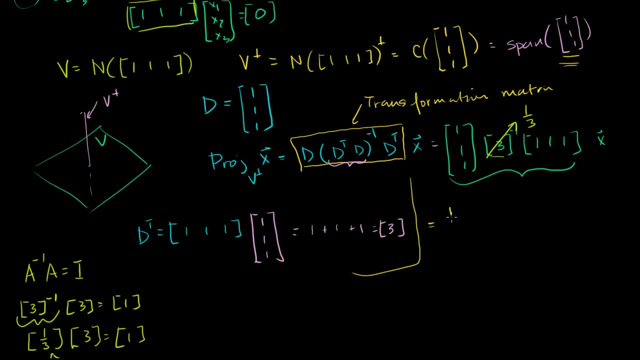 here This thing is equal to 1 third. Actually, I don't want to confuse you, Let me rewrite it So we get: the projection of any vector in R3 onto the orthogonal complement of V is equal to 1 third times the. 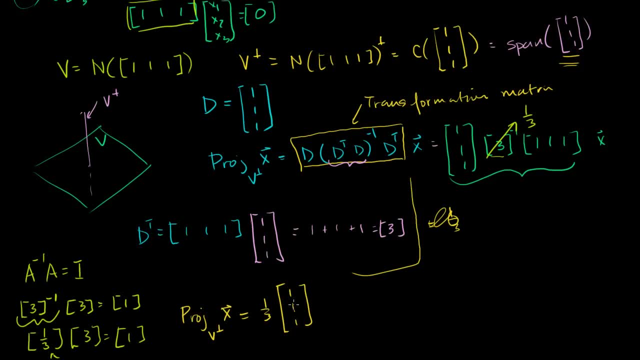 vector 1, 1, 1, times- sorry, it is a vector- or the matrix 1 on 1, times. that matrix transpose 1, 1, 1.. And then all of that times x, And you can see this is a lot simpler than when we did it. 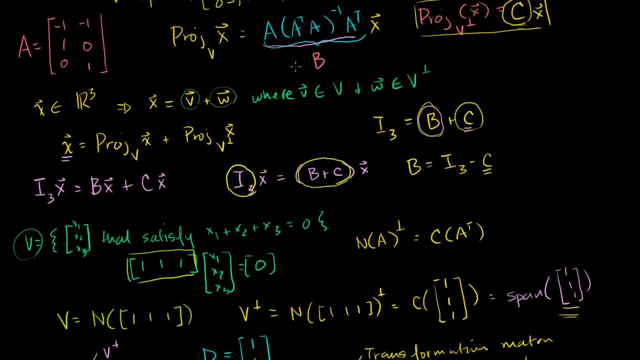 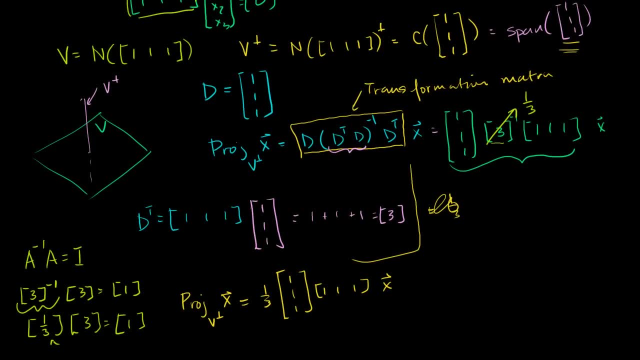 with if we had to do all of this business, if we did all of this business with this matrix. That's a harder matrix to deal with. This 1, 1, 1 matrix is very easy. Now what is this going to be equal to? 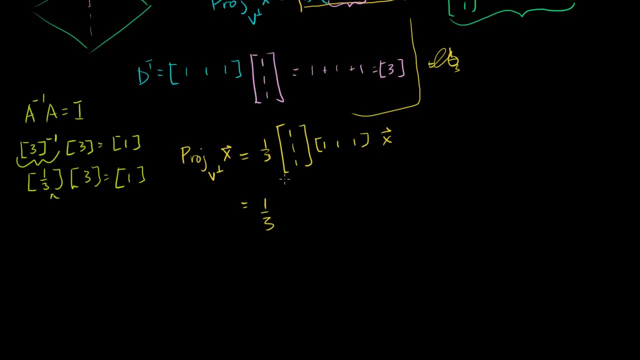 This is going to be equal to 1 third times. we have a 3 by 1 times a 1 by 3 matrix, So it's going to result in a 3 by 3 matrix- 3 by 3 matrix. 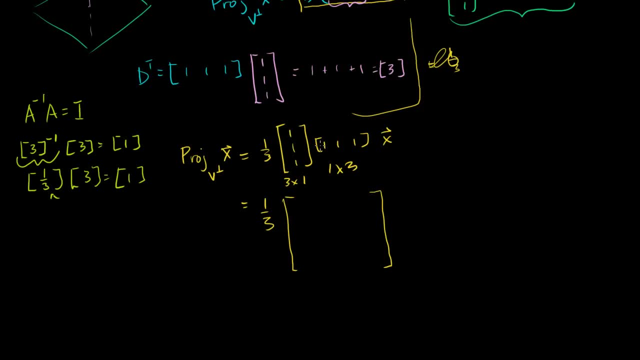 And what do we get? 1 by 3.. The first entry is going to be 1 times 1,, which is 1.. Second entry is going to be 1 times 1,, which is 1.. Third entry is going to be 1 times 1,, which is 1.. 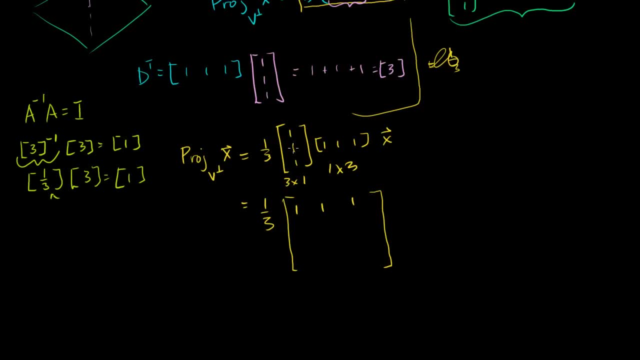 I think you see the pattern. This guy, the second row, first column, 1 times 1 is 1.. So this is going to be a 3 by 3 matrix of 1's. So just like that we were able to get that was a pretty. 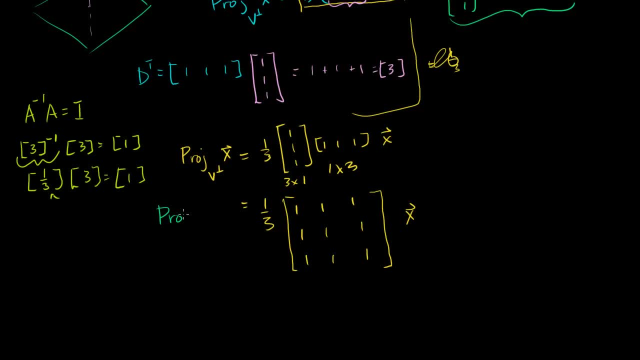 straightforward situation. we were able to get the projection matrix for any vector in R3 onto V's orthogonal complement. Now we just we know that this is our this thing right here. this thing right here is our original C that we said. 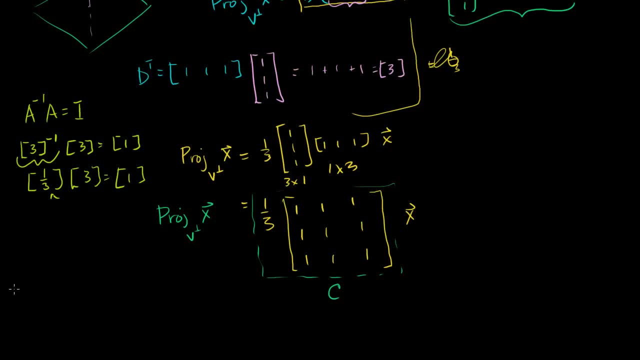 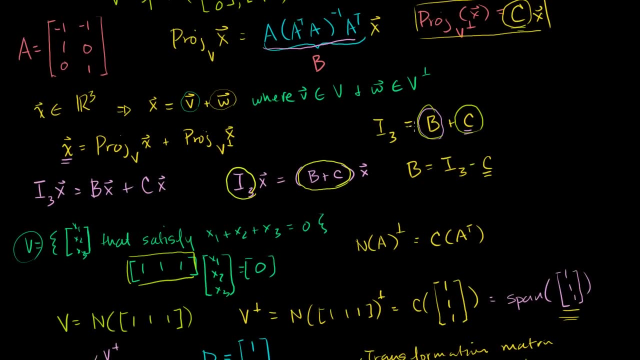 Now we said that we said that the identity matrix we wrote it up here. let me refer back to what I wrote way up here. We said: look, the identity matrix is equal to the transformation matrix for the projection onto V plus the 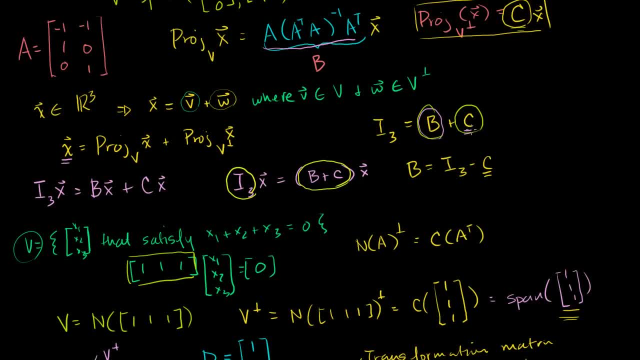 transformation matrix for projection onto V. So what is the projection matrix for the projection onto V's orthogonal complement? Or we could write that the transformation matrix for the projection onto V is equal to the identity matrix minus the transformation matrix for the projection onto V's. 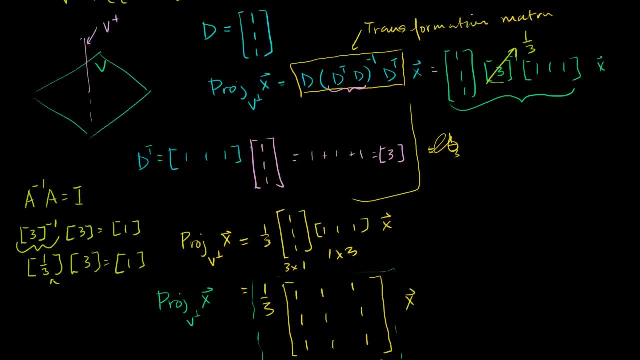 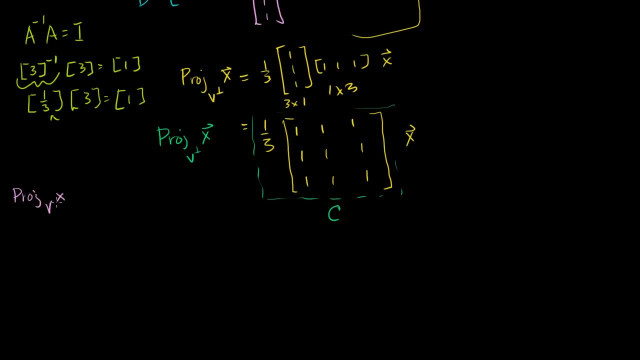 orthogonal complement So we can write: so: B is our transformation matrix onto. so if we say that the projection onto V of x is equal to B times x, We know that D is our projection matrix. We know that B is equal to the 3 by 3 identity matrix minus C. 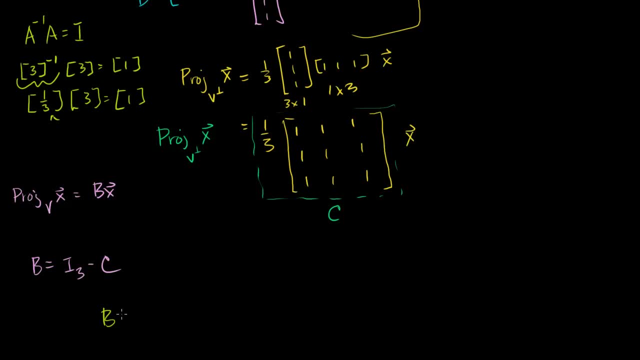 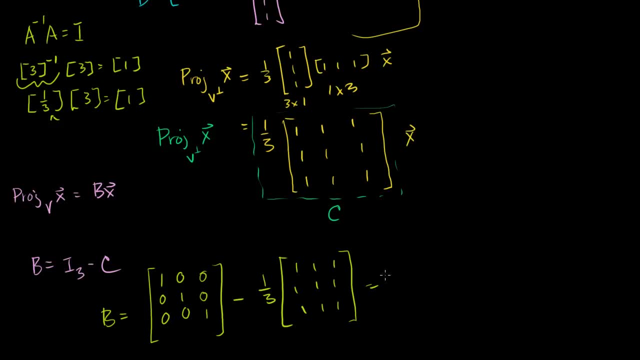 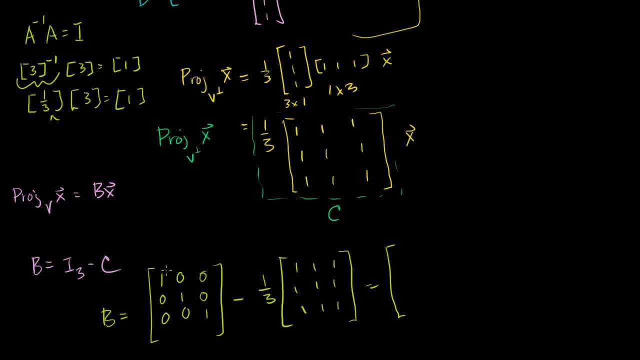 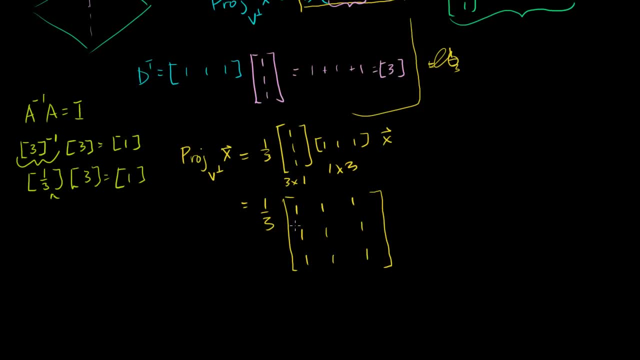 So this is going to be a 3 by 3 matrix of 1's. So just like that we were able to get. that was a pretty straightforward situation. we were able to get the projection matrix for any matrix, Any vector in R3 onto V's orthogonal complement. 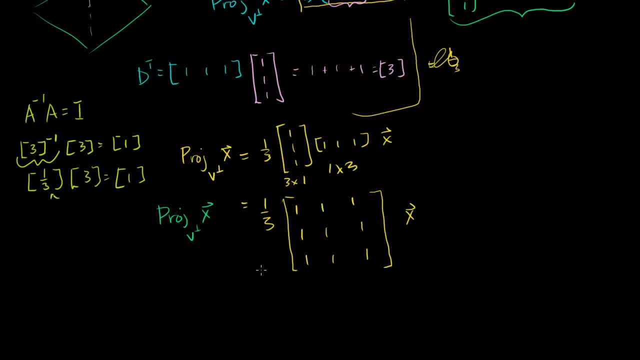 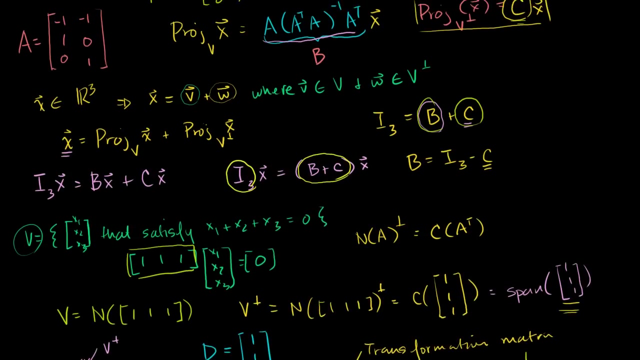 Now we know that this thing right here is our original C that we said. Now we said that the identity matrix- we wrote it up here. let me refer back to what I wrote way up here. We said: look, the identity matrix is equal to the. 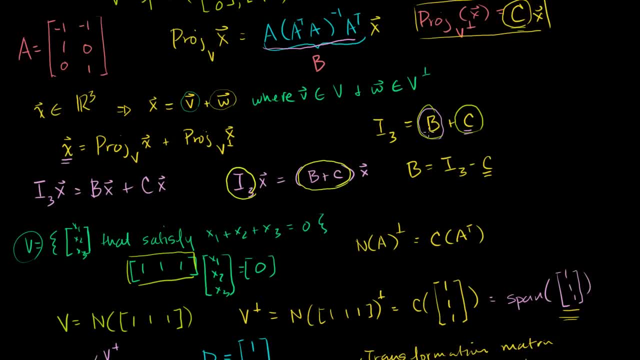 transformation matrix for the projection onto V plus the transformation matrix for the projection onto V's orthogonal complement. Or we could write that the transformation matrix for the projection onto V is equal to the identity matrix, minus the transformation matrix for the projection onto V's orthogonal complement. 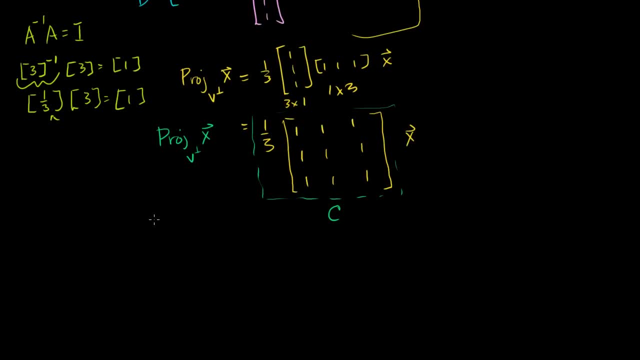 So we can write. so B is our transformation matrix onto. So if we say that the projection onto V of x is equal to B B times x, we know that B is equal to the 3 by 3 identity matrix minus C. 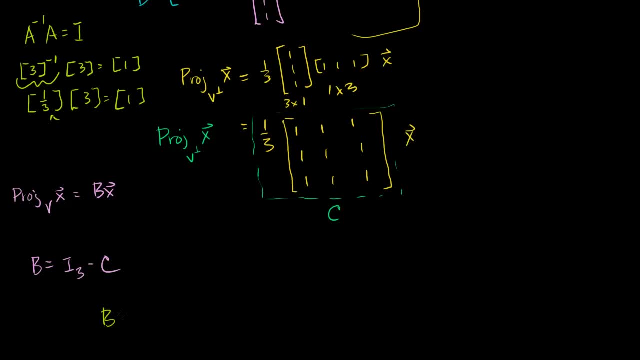 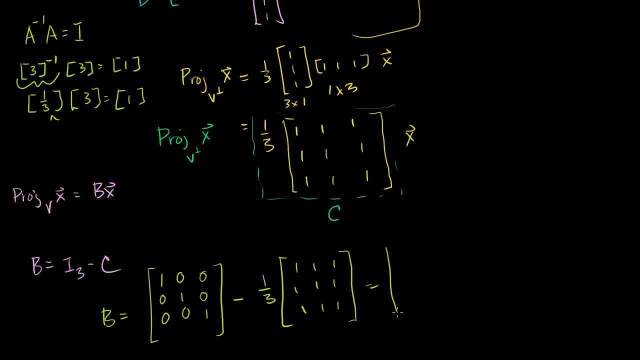 Just like that. What is this going to be equal to? This is going to be equal to: let's see, Let's, in our heads, multiply this out: All of these entries are going to be 1, third, essentially. if we multiply this out like that, 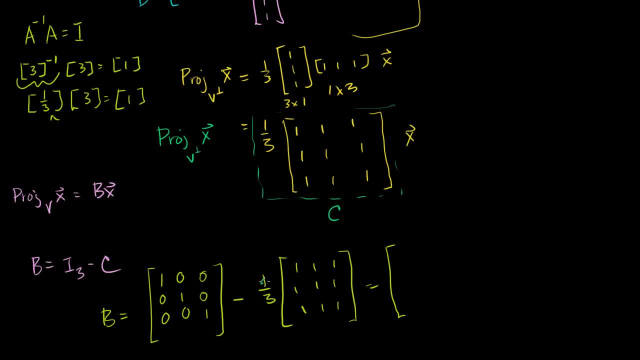